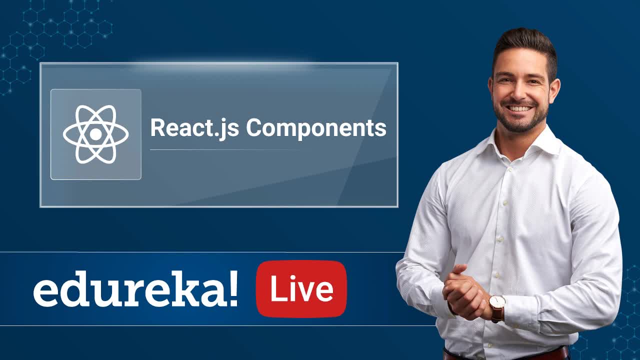 Welcome you all by Edureka. So let's begin our today's topic, that is, react component. See, guys, when we talk about any application, right, All application have four parts: front-end, back-end, database. And if I open this GitHub, let's see example. 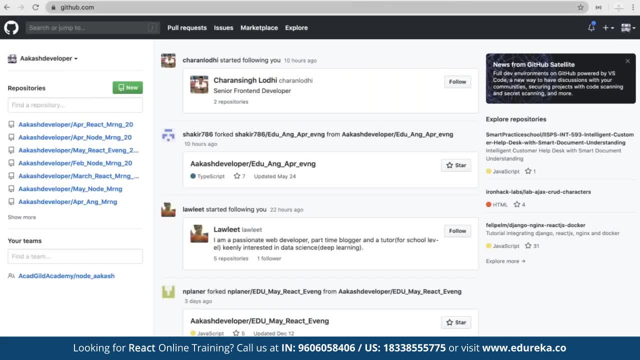 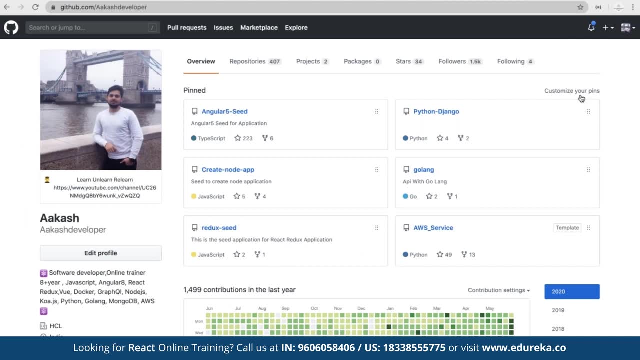 Over this GitHub. if you see, we have some front-end here, guys, right, The things I can see or the things I can interact with. the most interesting part of any application- right, The things that you can see or the things that you can interact with- is basically refer. 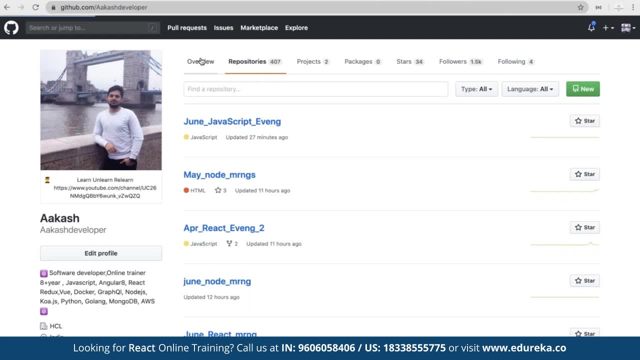 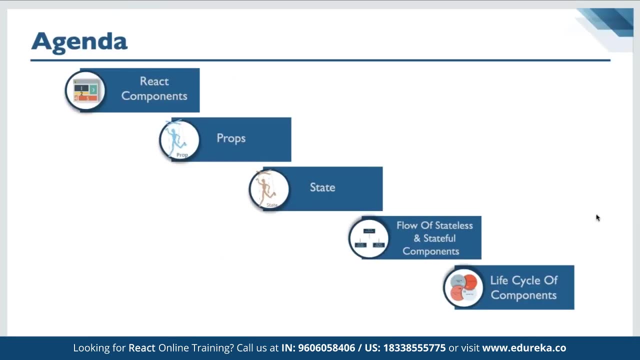 as the front-end of the application. Now what all data is coming on different, different tabs is coming from. a database means the things which I can see is basically refer as the front-end and the storage is the database. Now how exactly they both are connected. are they connected directly? 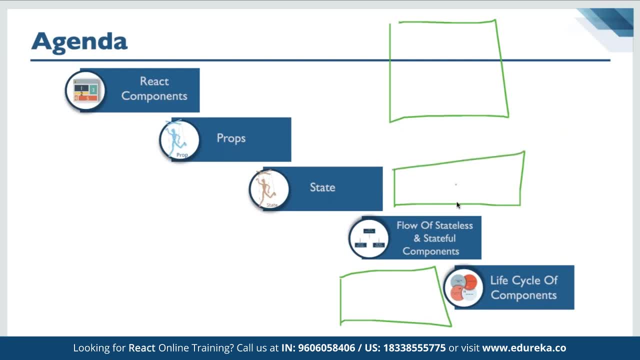 No, they are connected through the back-end. So the front-end, this is the database and this is the back-end. all the requests from front-end will go to the back-end. back-end will talk to the database and database will talk to the back-end and then back-end will talk to the front-end. 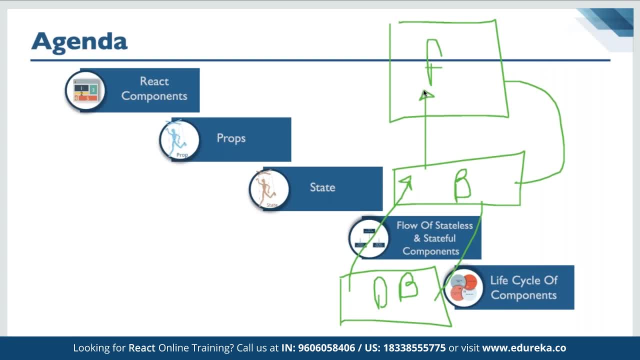 In short, whatever application you pick around you, You will see that every application must have these four part. fourth is a server will not talk about that today. So front-end, back-end and database, These are the three point three important thing that we have in any application. where exactly react, fit react? 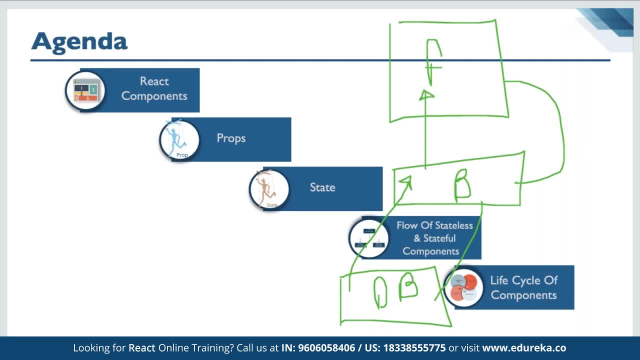 In the front end. So to display the content on the browser we use- react- and how we get that content. to get that content, We have to talk to our back-end. now that back-end can be anything like Java, Python, Ruby, Any back-end is fine. 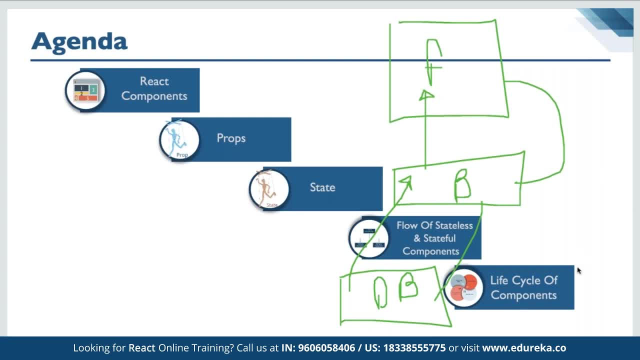 but ultimately at the end we have our front-end, front-end We'll talk to back-end and back-end will talk to database and we are working on the react as we have our- we can say- Front end of the application. Okay, so guys are agendas will talk about react, component props, state. 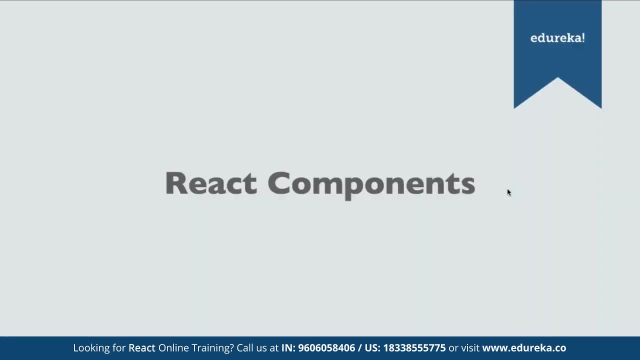 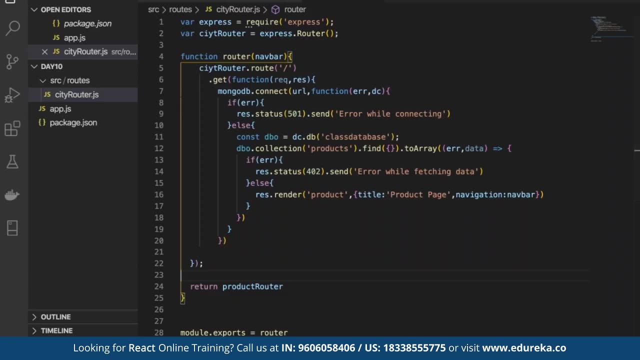 stateless and stateful component and life cycle of a component. I'll tell you one thing, suppose I'll show you one more graphic here. See, when we make any application right. Let's now stick to front-end, So I'll go to one page. 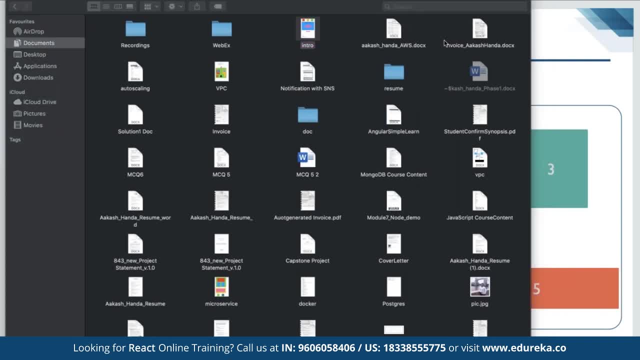 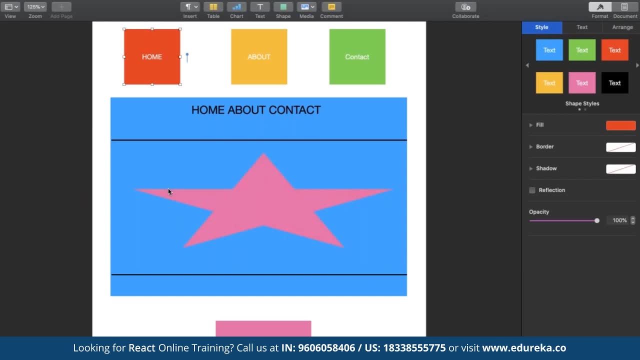 Guys, you must have seen one thing in your applications: That in every application We have something common. The common part that we have in our application is the lead. header and footer remain common application. So header and footer is, guys, something which is a common part of our application: the content: 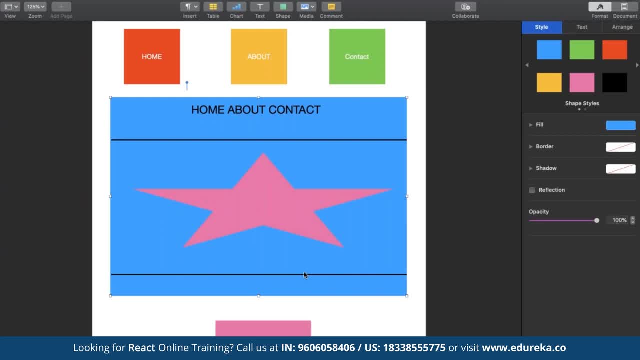 between the header and footer will keep on changing. So suppose if I click on home, the content of home will load in this area. when we click on about, about will load, home will go back and about will load in this area. when somebody click on contact about will go back and contact will load. 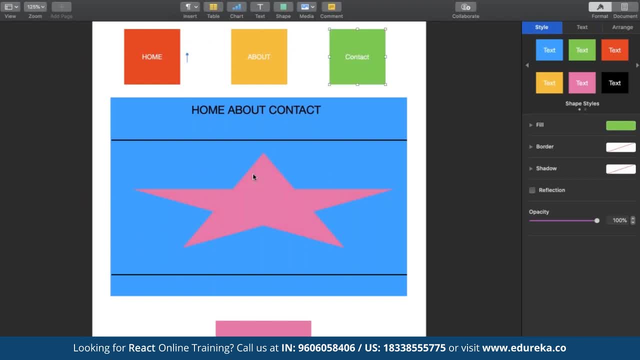 in this area. Basically, what is happening every time you're trying to switch a tab: the content is moving from one place to other place. in short, I can say that basically your content is moving, only is changing the replacing The part. it's not like reloading something. 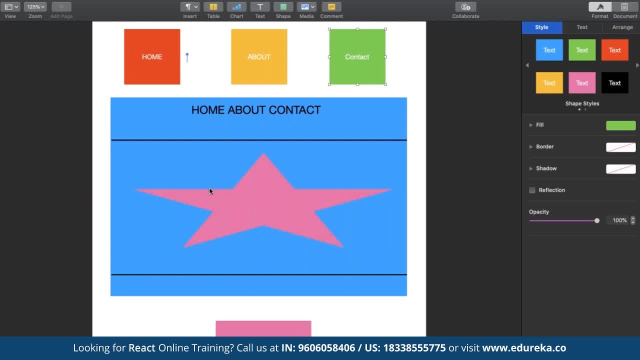 It's just trying to replace that part. Okay, Now, in this scenario, this called single-page application and this is called as your components. in this scenario, What happened, guys? the content will keep on changing, but page will not refresh. The content will keep on changing. 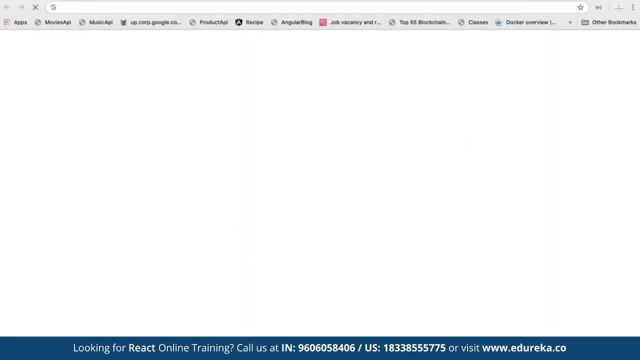 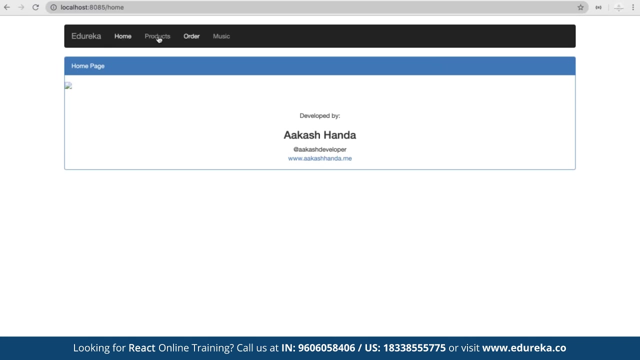 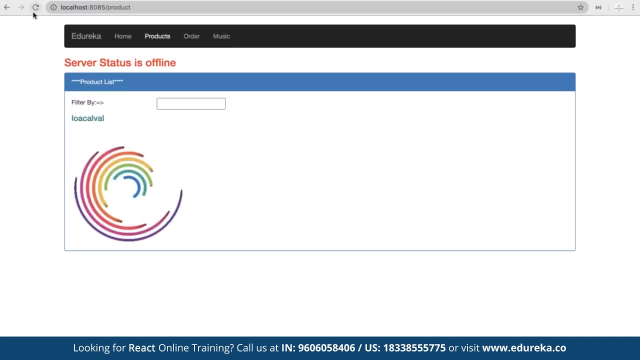 but page will not refresh. how exactly looking in real time. Let me give an example. See this website. Okay, over this website You will see one thing that I see: home product order and music. We jump from home to product. my page is not refreshing. 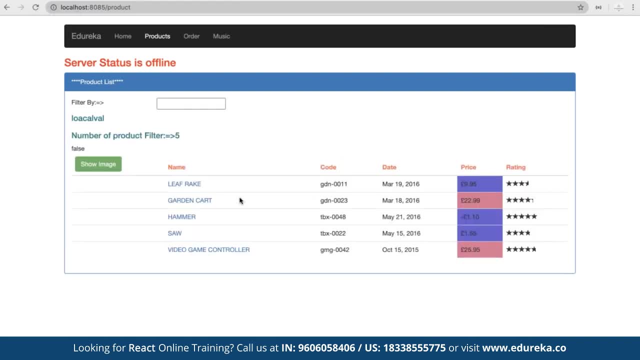 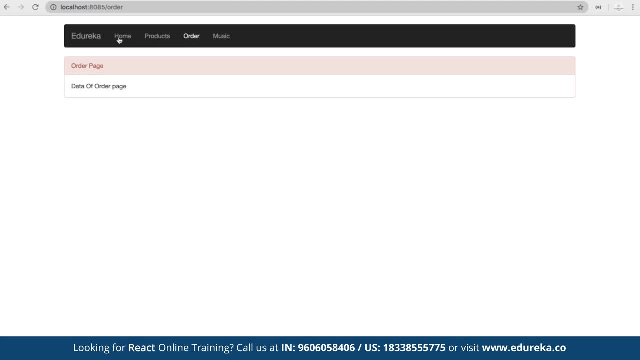 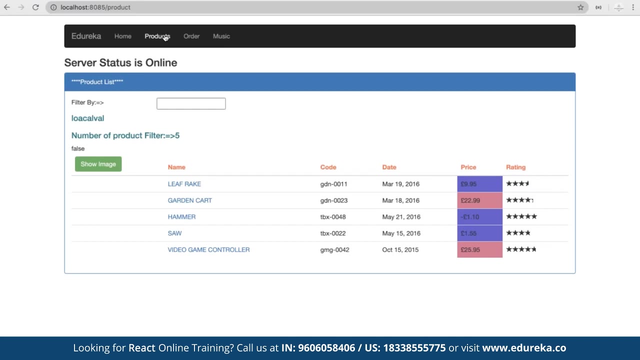 see the refresh happen here. My page is not refreshing but it load the content. when jump to order again, my page is not refreshing but it load a new content. see When I'm able to jump between one page to other page, but my content is only changing. the page is not at all refreshing. 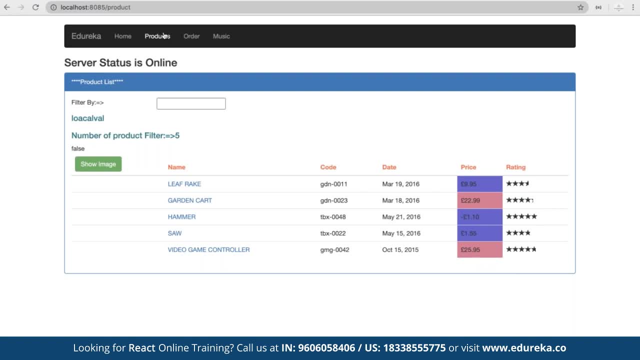 and that's concept called as your single-page application. in the single-page application, My content will keep on changing, but my page will not refresh, Okay, so in short, we can say that the content that we want to make right, the content that you want to make, will make them as a component. 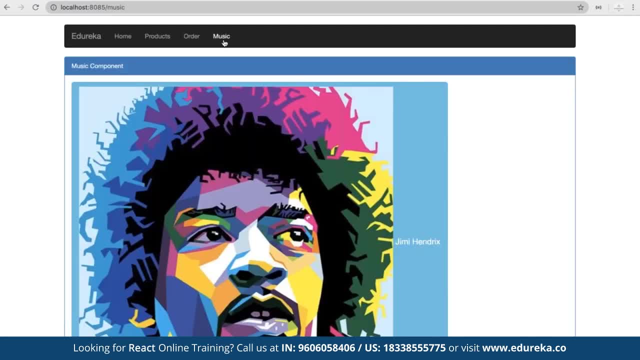 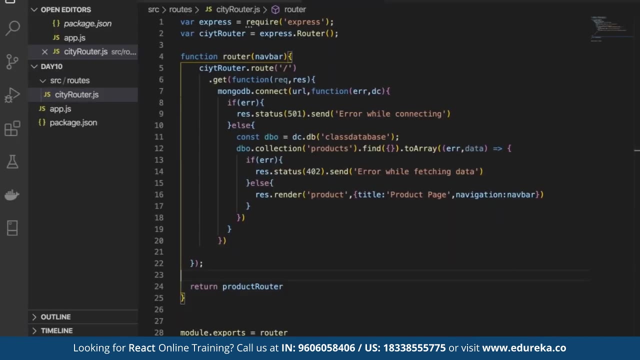 Each of them refer as one component. Each of them refer as one component and the content will keep on changing, but my page will not refresh from there. Next thing is, when we talk about this component now in a react, I'll open our new folder here and write some code for you guys. 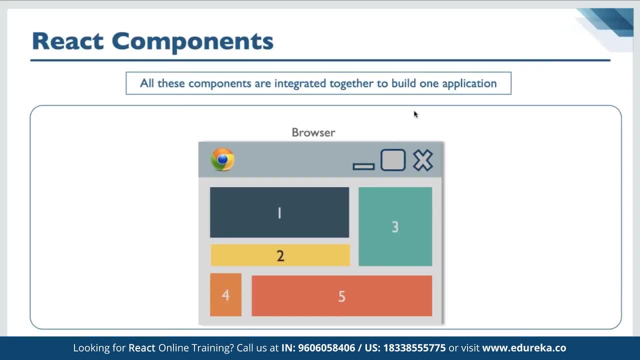 and text editor which I'm using is a visual studio code. Now, one component can be as big as your one header. It can be. one application can have multiple components and the data is coming from a back-end. It's like a database call. 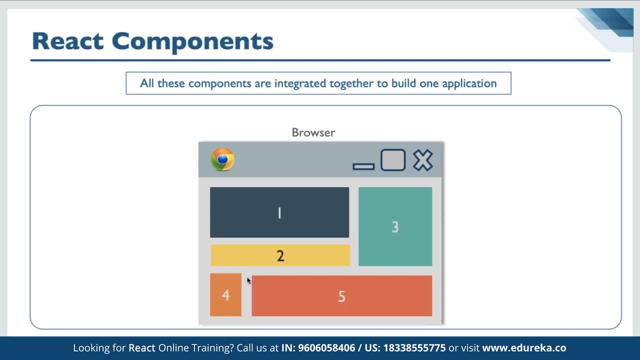 It's happening behind the scene in react and we're getting a data. So ultimately one page can have multiple component inside. that is like this: In all the page we can have one, two, three, four, n number of component, and one component can be nest inside other component. 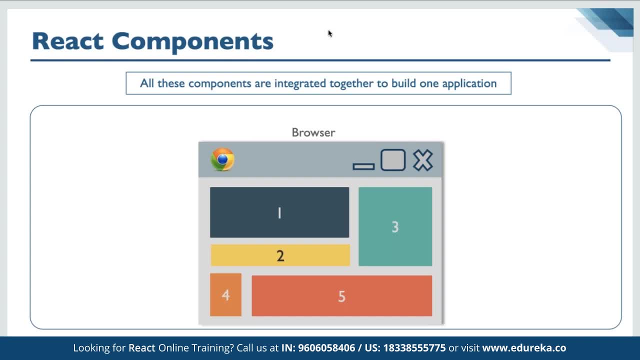 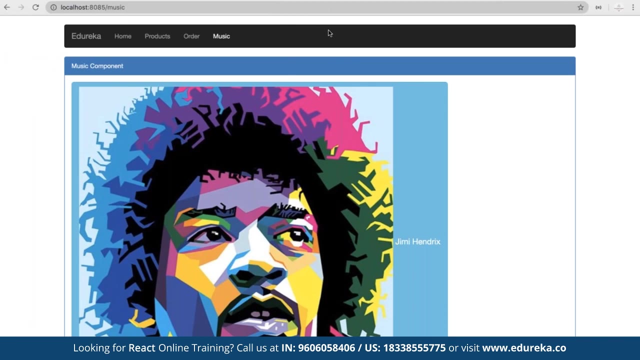 Also. it's also possible that you have one component inside that we have other component means we can have nested component Also. we can have an individual component also and we can have guys nested components also. So in short, we can say that we can nest any component anywhere in my application. 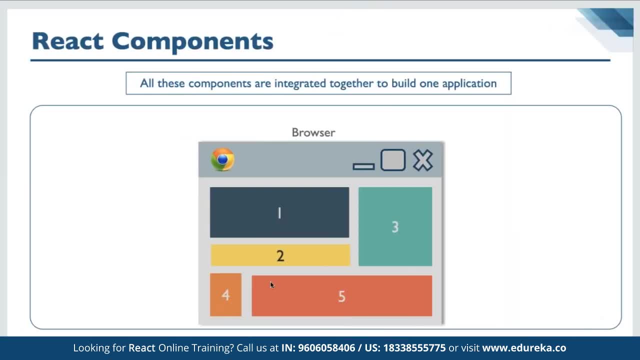 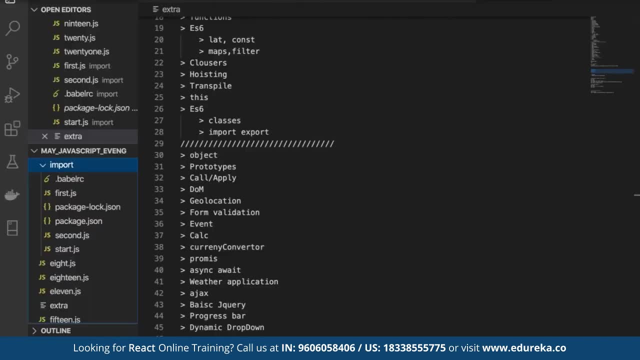 Now, if I go back and I make a folder to show the example for this world, I know comments are available and then you can come back to a PPT and read more about that. So let's close to things So we can easily update a change, the component. 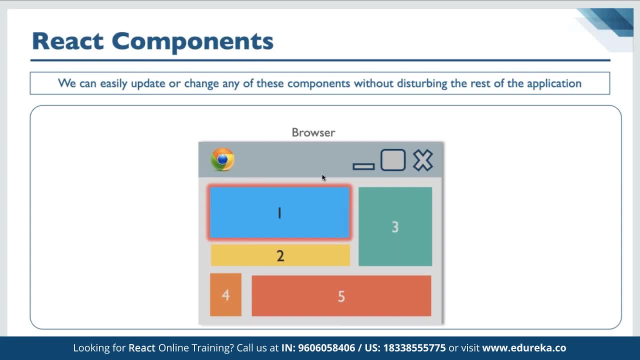 without disturbing the rest of the application. The best part of the single page application is that the company structure is suppose I want to make some change means a page. Suppose somebody click on button I want some, some content there, so I can change that content very easily in this space here. 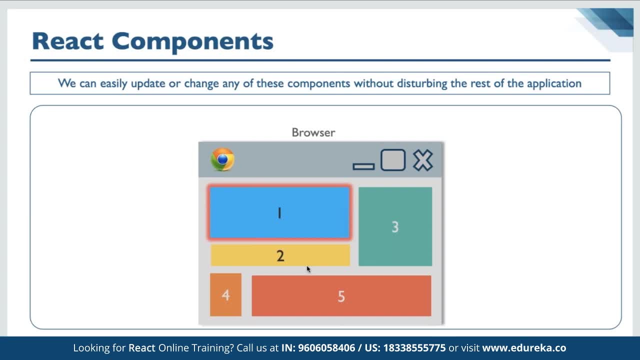 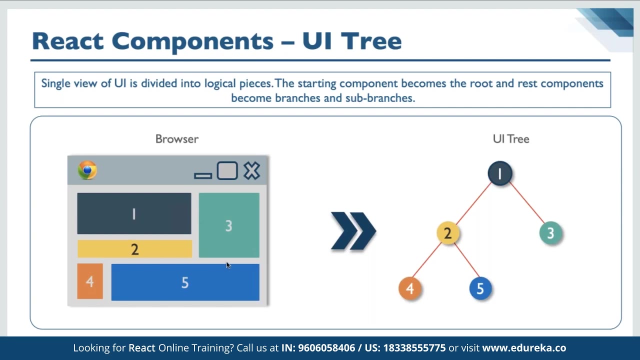 or here or here, and without changing my whole application, Without refreshing my whole application, I can mean that make the change where exactly I want, instead of refreshing that. So it's make a view is divided logical pieces. They all act like our logical pieces. 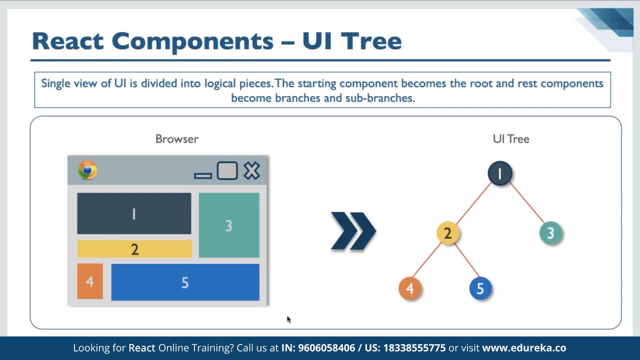 We can have one main component and we can have them a child component. main component is a one that nest all my other components like that and then we have a child component there. So a starting component become the root component and become the branch of subcomponent. 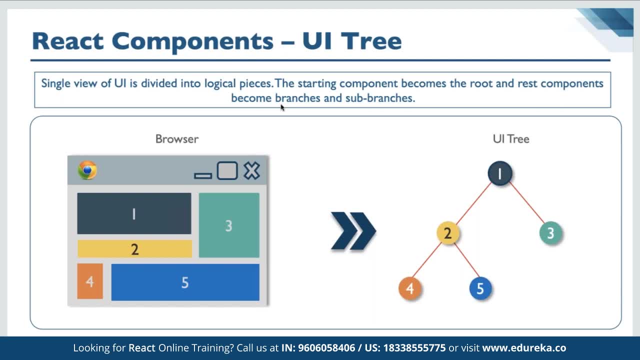 I said that it is possible, guys, that we can have one component and then we can have more than one component. It means one component can nest n number of component, or we can have all as our individual component. Now, next, let me show you what all different kind. 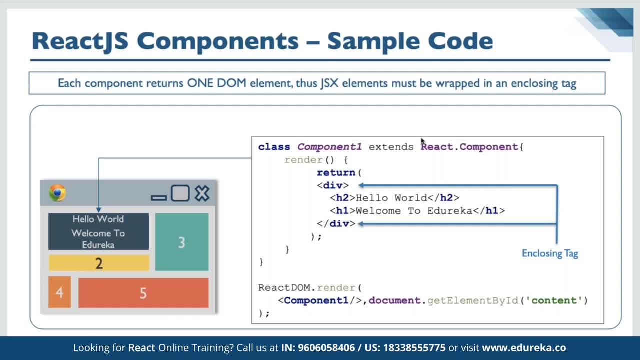 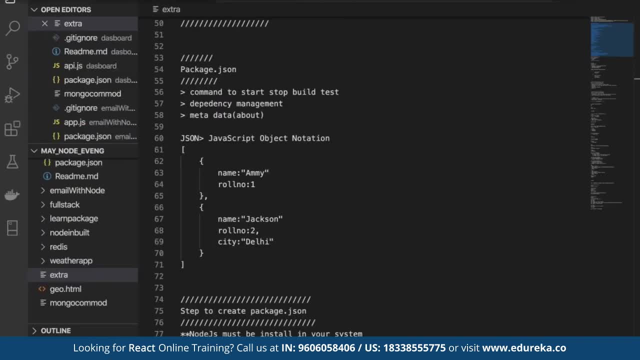 of companies are available in react and let's start drawing some comment for us. for doing that, I need one folder structure for me where I can write some content for you guys. Let me do that. I'll do something in a more practical manner in each application of react. 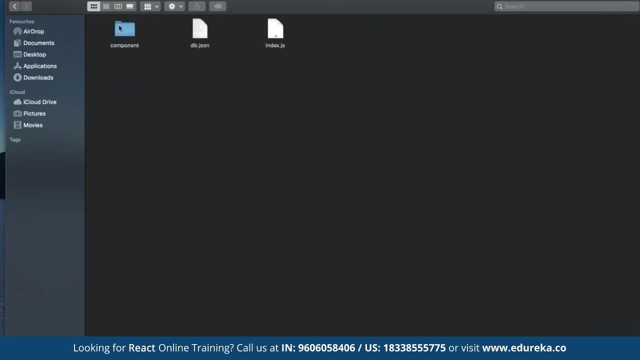 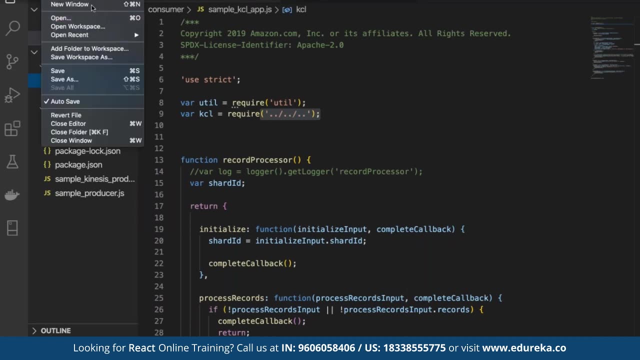 You have one thing called SRC, SRC. in the SRC We make a component. So let me start from beginning of fitting a component. I'll make a one text editor. I'm using a visual studio code. You can go with any text editor of your choice. 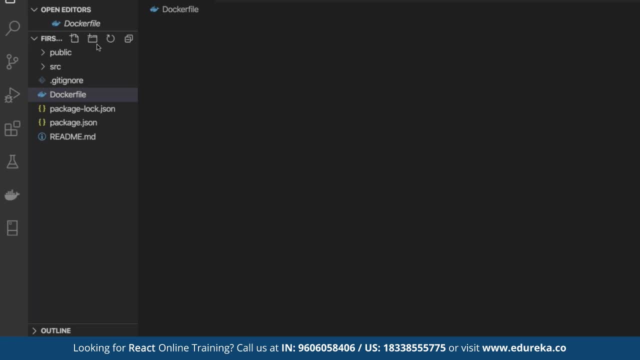 And then I'll make a one extra file here first of all. So I'll give you an extra file here to give some zest of this thing in the react. basically a multiple way to create a component. What are different way of label to make a company. 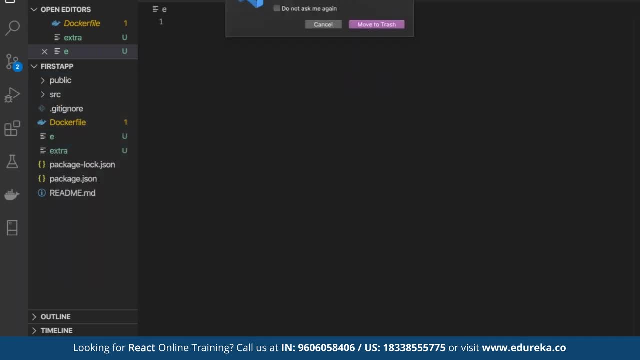 Let's see that first, guys, in react We make a competent by three ways: One is called as a class component, class component, and one is called as a functional company, One is called as a class, one is called functional and the one more way that is called as your hooks component. 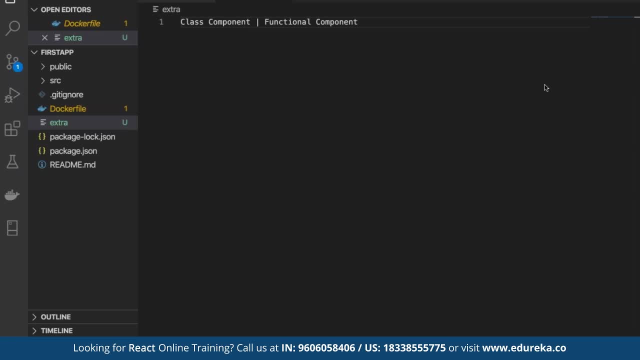 How are you? We are different from jquery, is very much different. So jquery is a library, is a proper structure, oriented structure. So jquery in lab react and no comparison. So, guys, a component is divided into the multiple part, like what is called class component, functional component. 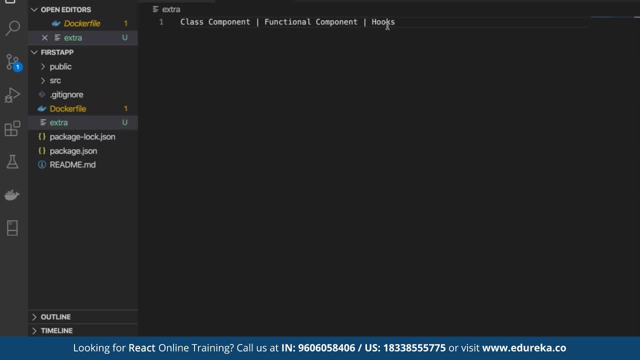 and hooks component. hooks, component are the new way to create a component. Okay, folks, company. Now what is the class based component? and functional company We just talk about to, not the hooks. today, What are the class based component for the company? The class based component is basically refer. 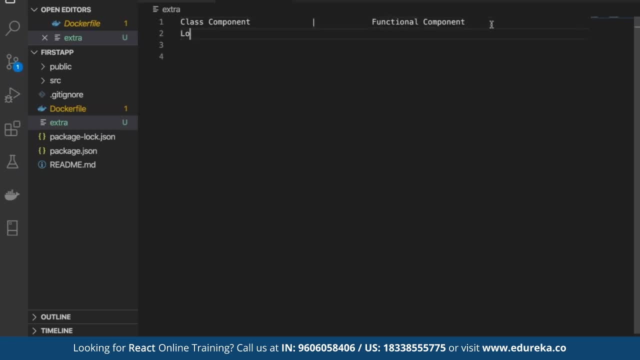 as the logical component. logical And the functional component is basically refer as your display component And even we can call it a dumb component also. So class based component are the logical component, whereas functional components Are basically called as dumb component. Okay, so logical component, basically all your logic. 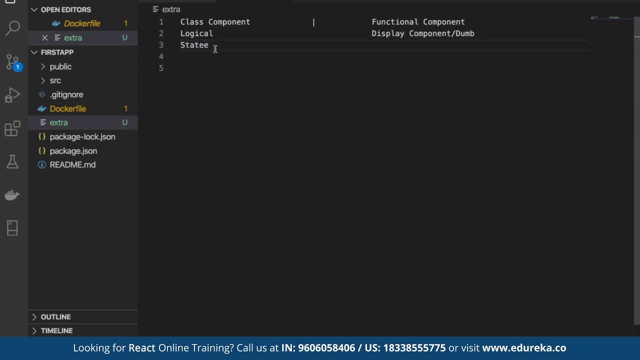 It can maintain the state. I'll tell you what is state in a while. and it cannot maintain the state. Cannot maintain the state? Then next thing: class based components are also called as your stateful component because it can maintain the state, and they are basically called as stateless component. 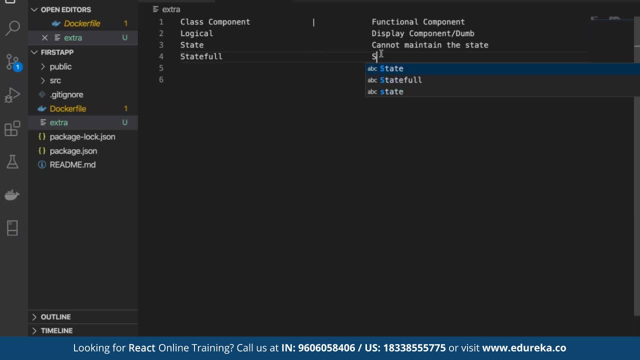 So how exactly in real time it work. State how you just do. we use only one kind of component, both, both kind of component, basically in one application and use all kind of components. how suppose any your API call happen? All your API calls will happen in that class component. 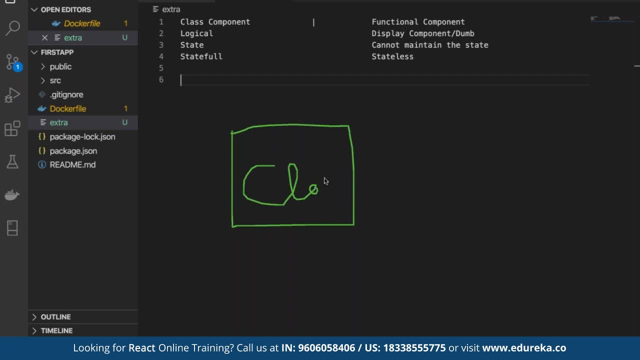 Okay, in the class component We'll do all our API calls. Now it get the data, Now ever display data. So we kept it for a logics and the data we got we pass to our next component, called functional component, because they are light in weight. functional components. 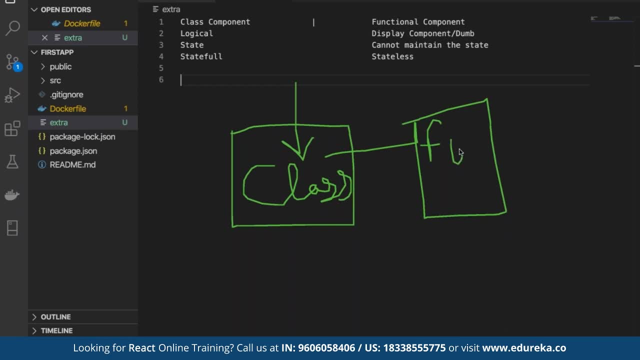 are light in weight. So, as in the react there, nothing like your HTML is different. If I and the CSS a different file, CSS can be different file, but HTML and the logics are not a different file. Basically, HTML and JavaScript are written together. 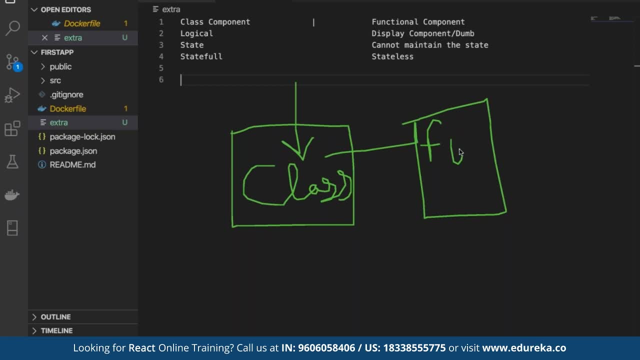 in a one single file. We call them as a GSX. also your HTML and the JavaScript written in one single file. We call them as the GSX as well. So basically, all the logics that we built in a class will be the component, will do in the class all my API call. 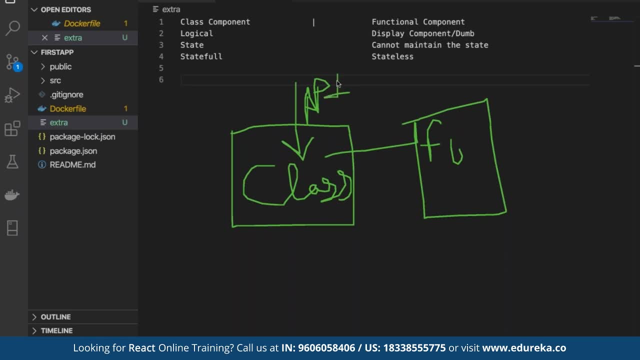 I'll do all my data interaction I'll do, I'll do in my class component and the data which I receive I pass to my functional component. So functional component act like a display and the class common act like a logical component. That's how these two common are different. 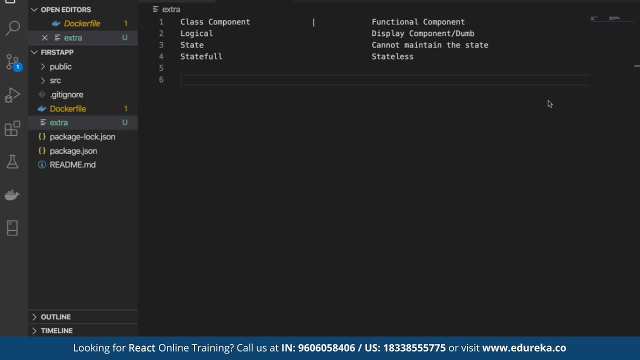 So, guys, let's start drawing. are both the component there? So first of all I don't pick a pointer. So in the SRC I want folder called component. I'll delete this folder. Basically we have one main component call your index file index. 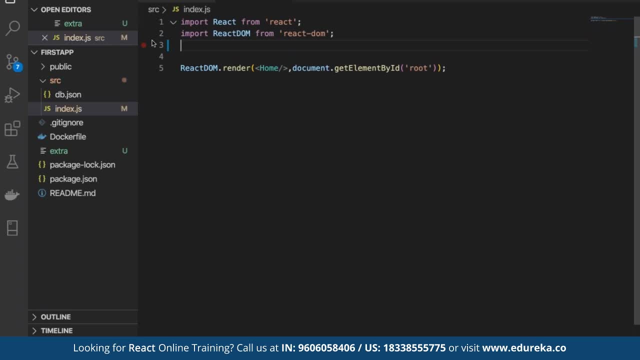 act like my main component is the starting part of the application and it act like my main component, index. Now I can make a multiple component in one application, So I'll call one folder component In this. I want comment by the name of homejs. 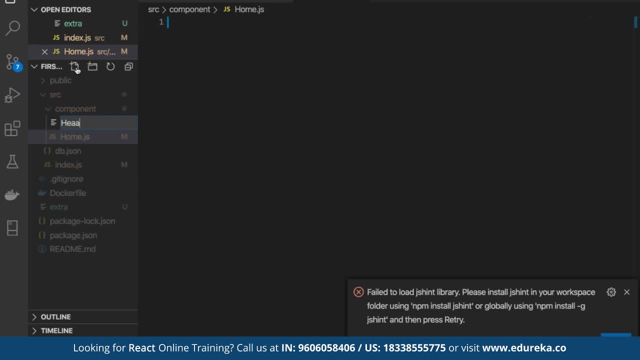 one comment by the name of your headerjs and one comment by the name of your footerjs: home header, footer: The component, now one I'll make a class component to. I'll make a functional component. I will decide it. they decide, in a way, the comment. 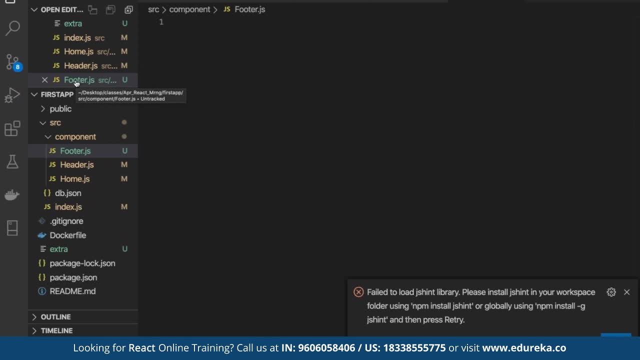 that is going to call the API, or the company, which our logics part. call that as a class and the component, which is just for this to the content, call them as a functional. Now let me show you how exactly it look like to make any component. 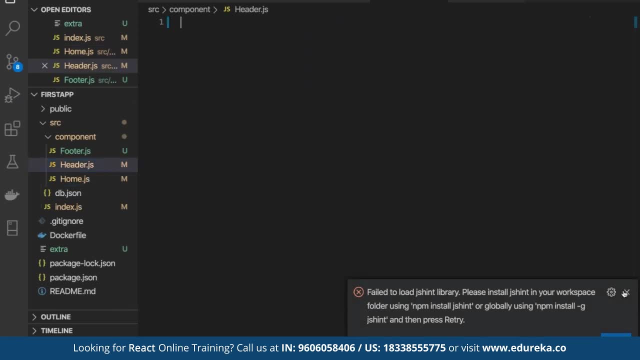 First of all, let's make a functional component. to make any company in react. You have to import one thing called react- React from react. The very first thing you will import is react. guys react to the one library and we import it in my application. 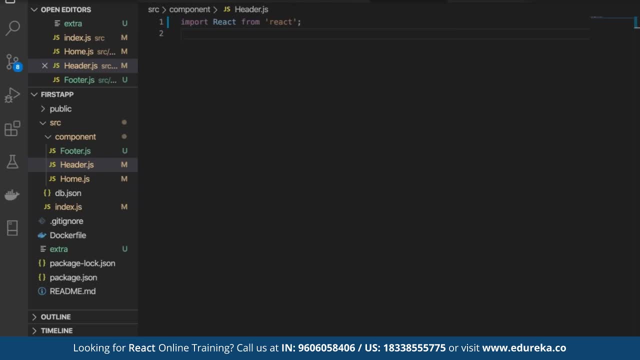 so that I can use it. So first step is you have to import react from react always in every component with my class or a function. Then after that we give a name to my component. How we give will say: const home Equal to bracket arrow, curly braces. 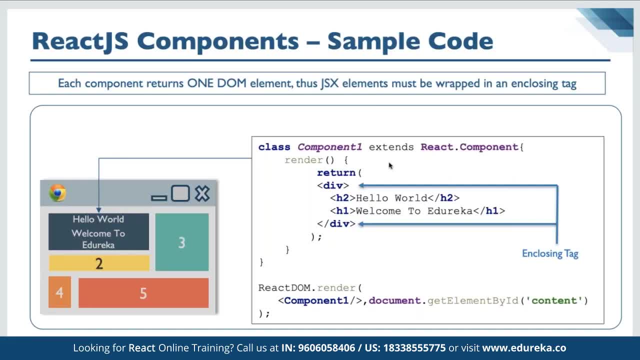 We go back to our PPD's also. one second See is showing an example of class based component. So we'll make personal functional component and then we'll come to our class based component. Every function that you write will return something. guys, I'll return one day. 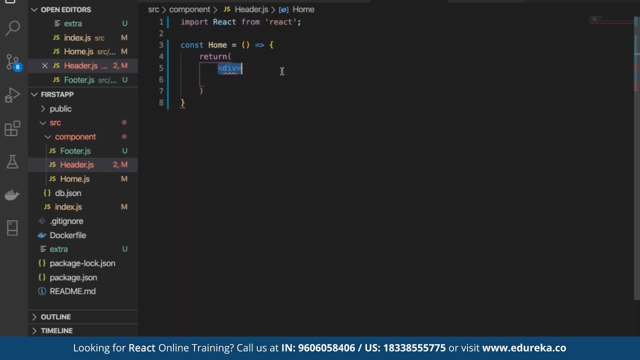 A lot of things are there: Dave, header, footer. So first of all I just return one H1 time In this H1 I'll write react, react, edureka, Edureka. then every component that you create, you export that component, export Default, or export that comment by same name. 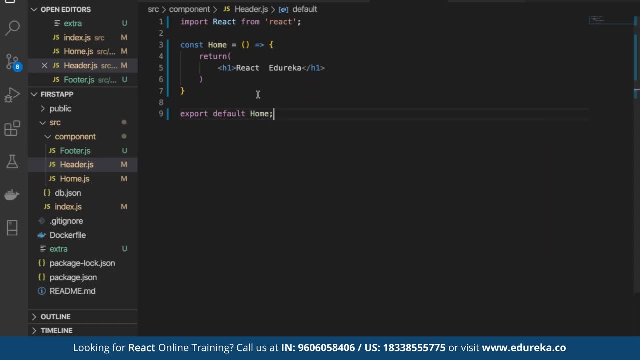 Now next thing, we take this home to my index file, index to the main component. that will display everything I'll import here home from possible. I just got a header right. I went wrong name here. Sorry my mistake, It should be header. 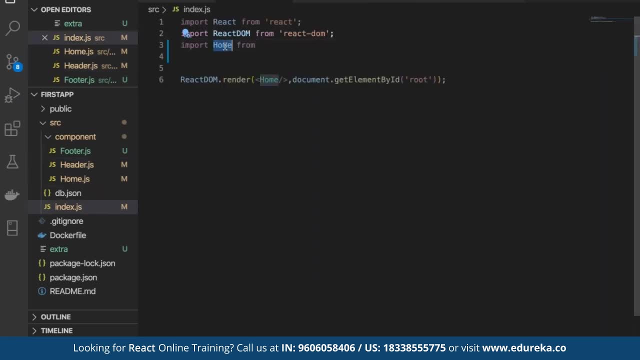 I'll take this header to my index file and import, like this import header, and give the path of the file that is, slash component flash home and this header I'll put. so, guys, first of all you have to create a component, export that and display in the index, very first step. 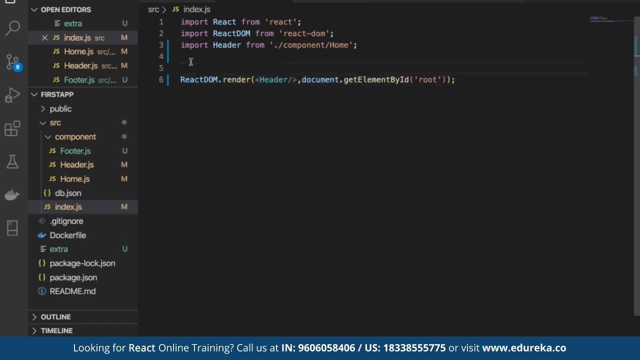 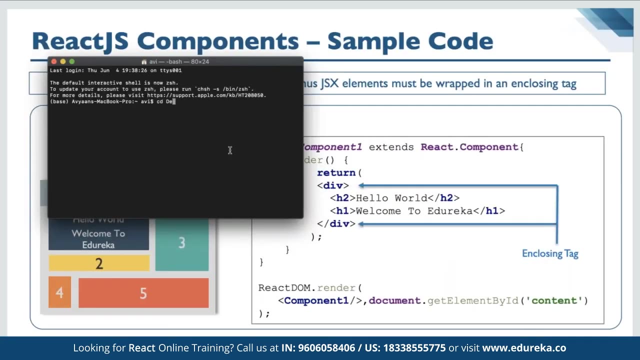 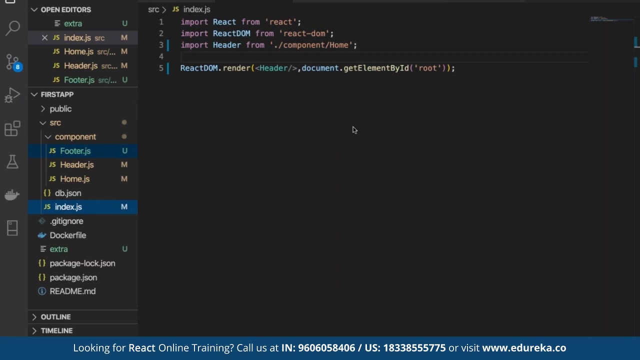 but the multiple step will proceed for one by one. now To run this application You have to go in this folder, So I'll go into the folder CD, next of classes, and then the folder name is on a folder name. Very, it is there. 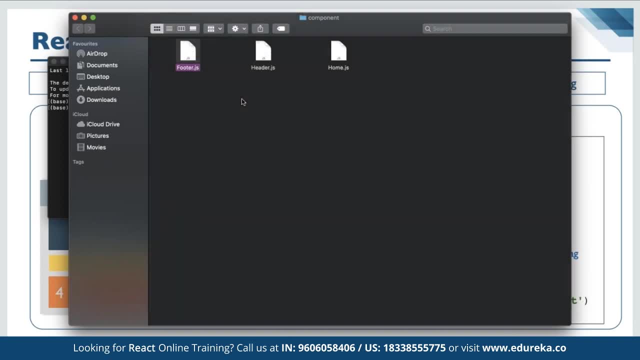 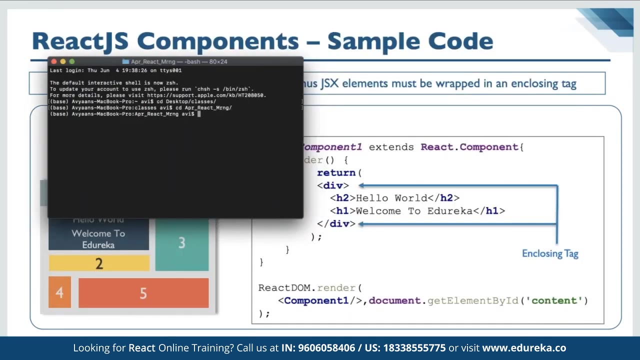 So I'll just check the info. Either folder that we have picked is react morning and I think we're dealing with the first happening. Yeah, so I'll go into the folder CD- react morning pasta. to start the application, go inside the folder type and pm. 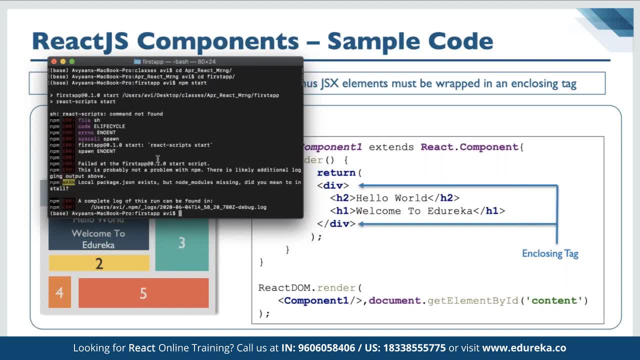 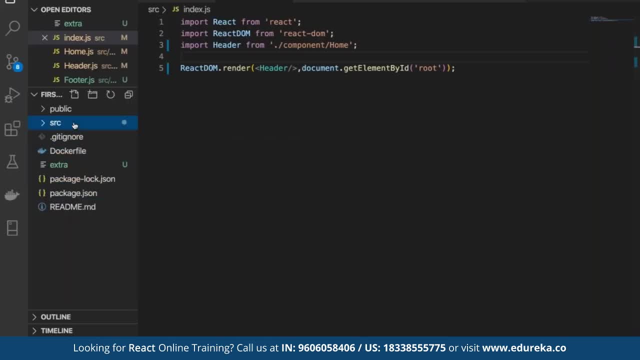 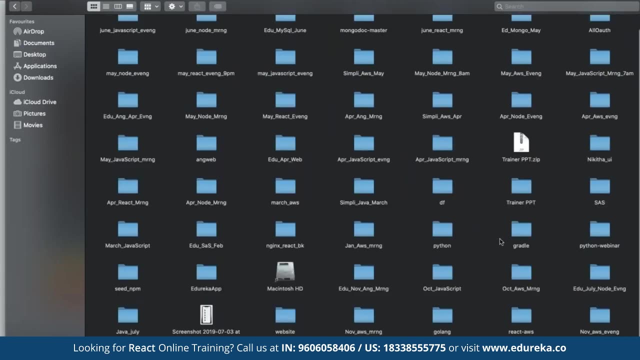 Start address. I'm going to write folder. Oh, I think in this folder my node model is they not there? Okay, Okay, Okay, Okay. but it is not run because my node module is not a part of this folder. I have to get from the other folder to that. 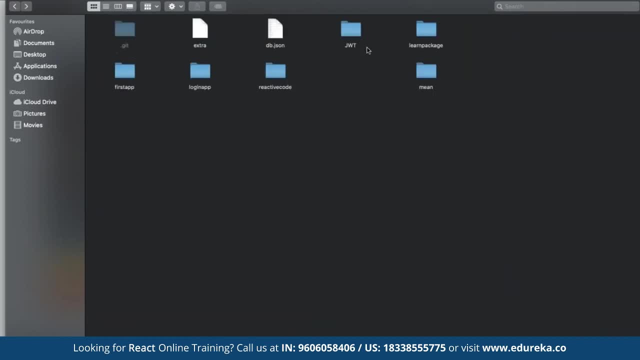 I'll just copy the component which I've just created for the reason, so that I can use it. So my folder Is the one. this is the one I'm using. I'll just pick this component folder here which I've just created, into the folder. 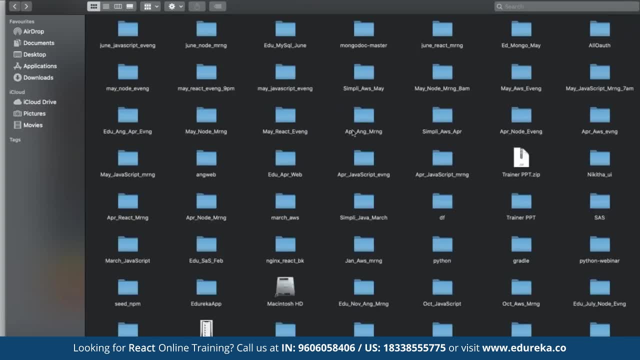 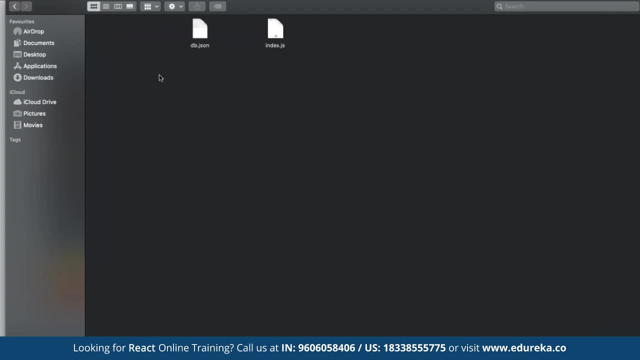 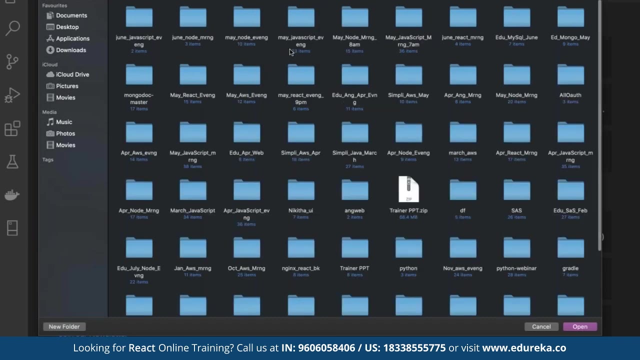 There are no more because I don't want to waste the time in setting up the application in my system right now. Yeah, we can go with this one. There are need the component and make it, and the folder name is reactive. So we go to classes and that is reactive. 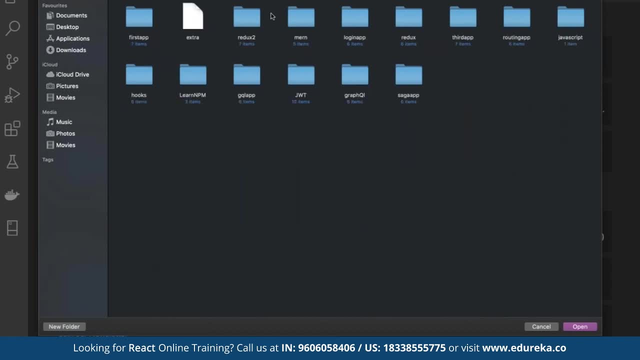 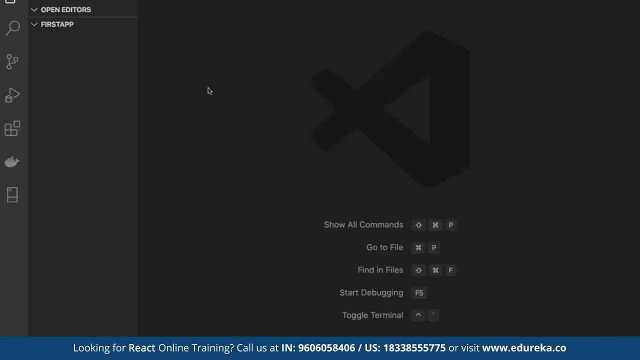 A folder which I'm using is and that particularly first app, and I run this application now and I'll make a one more change in the application. We'll just take a compound folder In the index instead of a home. first of all, whether I enter the header is matter of combine. 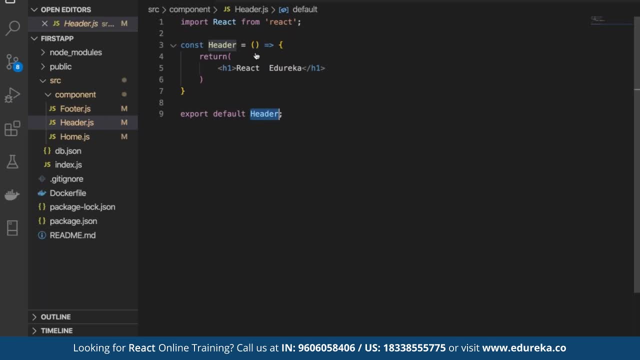 I want to show on the screen. So let's take it, Let's go to index, Let's import it and display it. now Let's run this. run this application running. I already told you. go inside that folder and write npm- start. 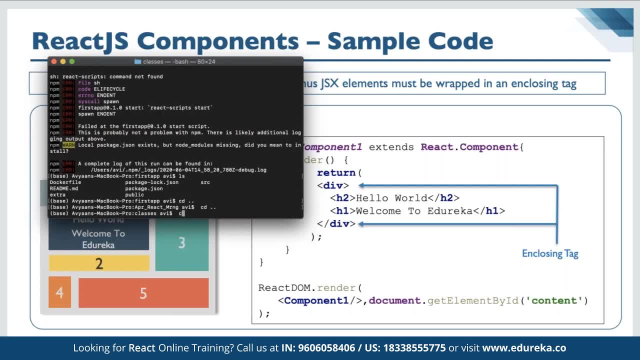 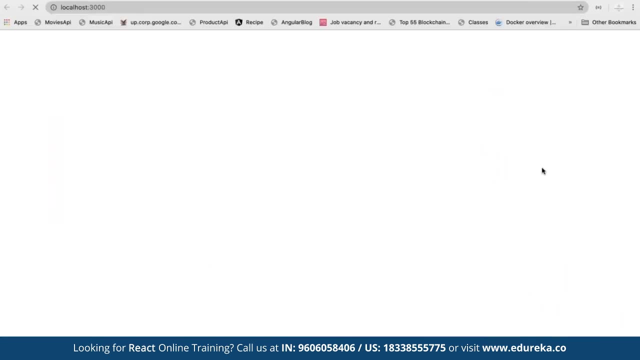 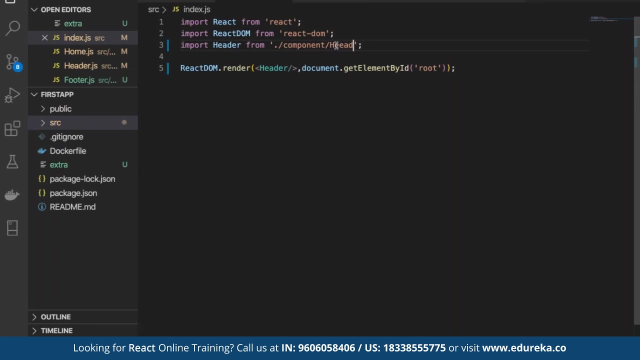 That's it. CD dot-dot, CD react evening pasta and then npm start By default. it run on the port number 3000.. Let's run it Now. we got one. You have imported the header. Oh, there's no another component really feels fine. 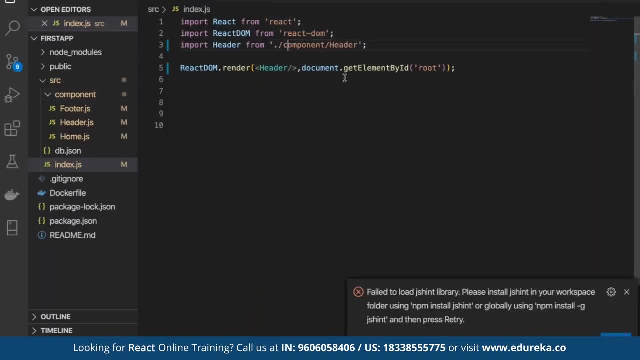 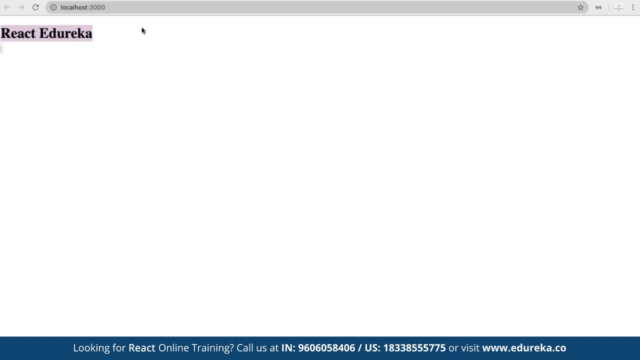 We import from components. He's a small. I had a capital. There's a case sensitive, I'll see. So, yes, we get the gap and Erica. You see the art editor Now even make a change here With the react and Erica webinar. 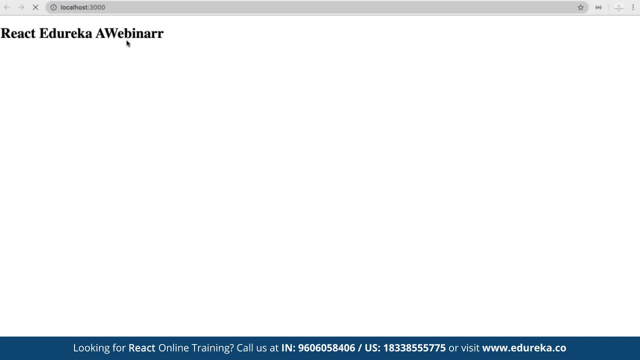 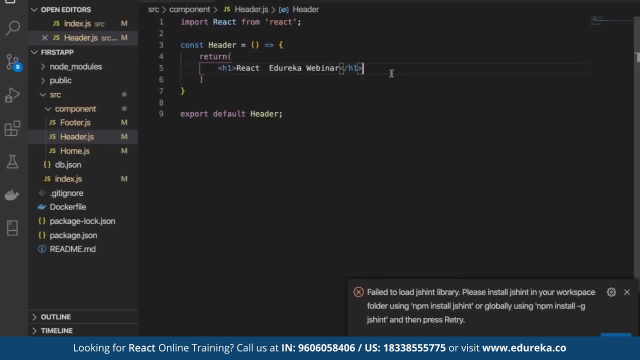 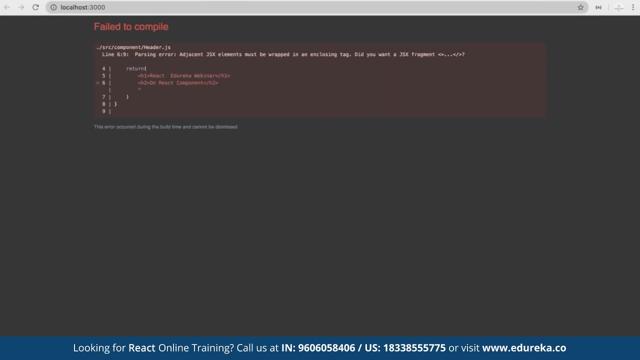 Like this. I'll go back See it become react Erica webinar. So I make one header. suppose I write one more s2 tag. We'll say on react component. Let's see what happened. It threw me the error Why there is this is a basic fund up this called GSX. 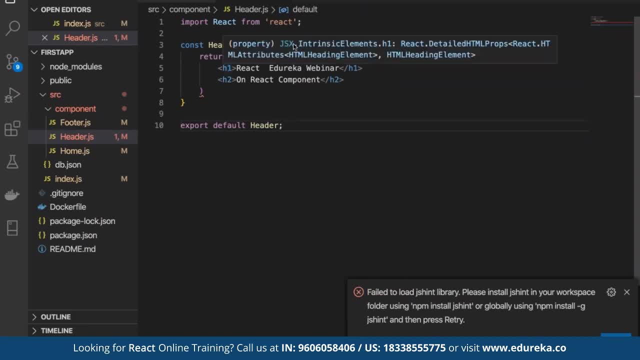 See my over over that you'll see GSX, The basic funder of the application. You cannot have more than one tag like this. If you have more than one tag like this, you have to wrap them into some parent element. It can be div. 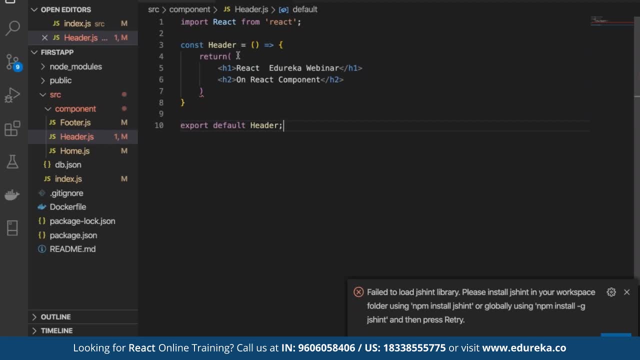 It can be header, It can be footer or react. Give us one thing called react dot fragment means if you have more than one element, Okay, you cannot return like this because of the basics structure of a JavaScript. Yeah right, react dot fragment. 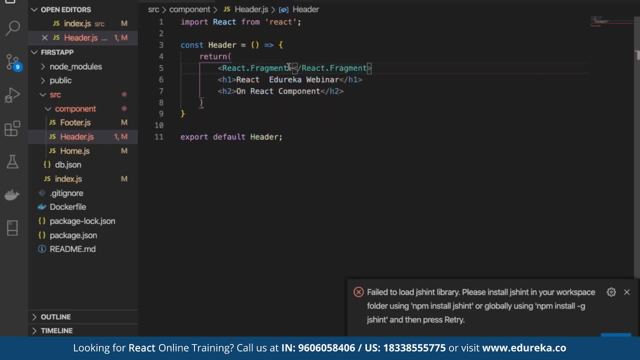 The one tag, the react, give us just to wrap them into one, Just to wrap them into one so we can wrap them into react dot fragment. Now we go back, we can see both. So I'll do one thing: I'll make a one h3 tag here like this one. 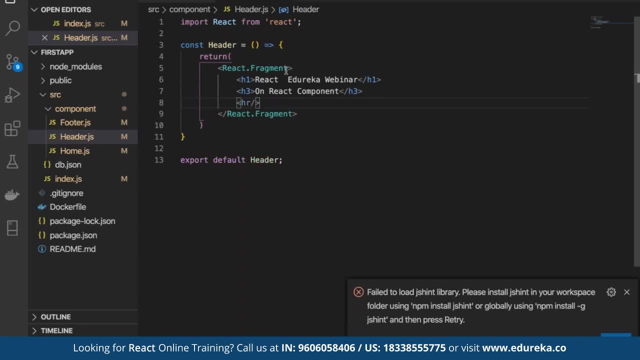 and under that I'll make a one HR tag horizontal line and I'll put this content in Center. So it start looking what will make up application. That should start Look how good it is of component Center And this Center. See, start looking better. 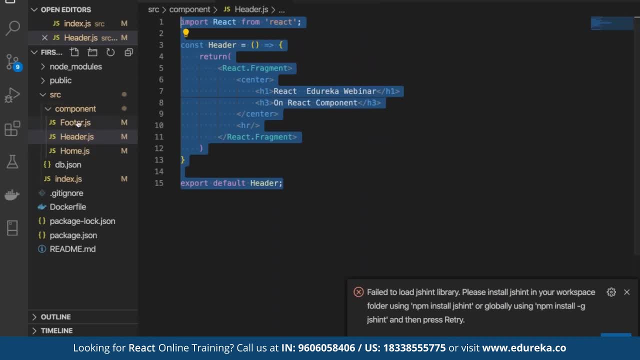 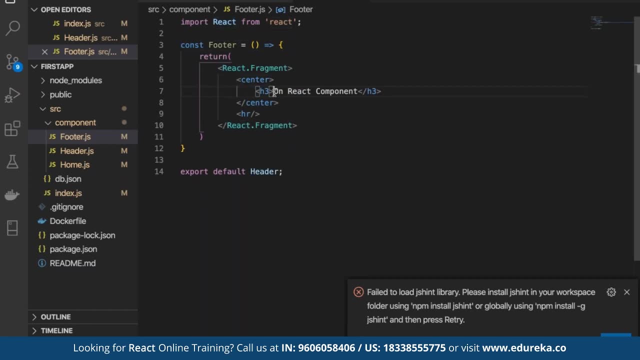 In similar fashion, I want to draw my footer also. I'll set footer At the rate. I'll take a h3 tag. I'll say ampersand: copy your copyright symbol: Edureka, It's a footer. now. next step is: 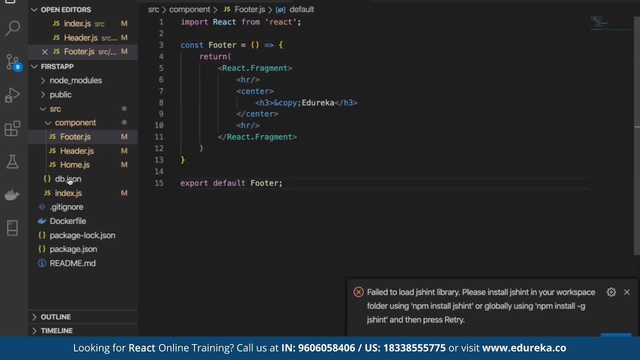 to export footer. there's now from my index, only one component we render, always from index, Only one component we render. Also, all are my functional component. I'll make a home pump Now. what I'll do is because now I need to render the footer. 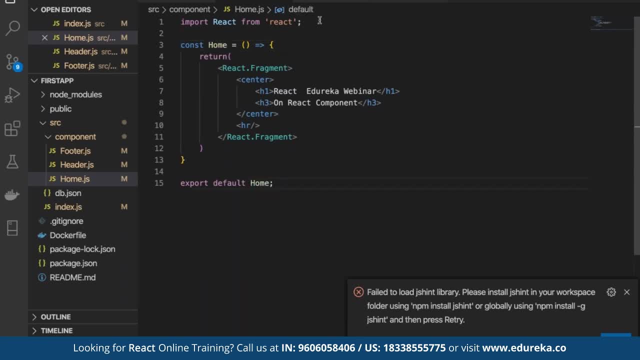 Also header, also home also. So I'll call my header footer directly here. I'll say: import header from Dot slash header. similarly Import footer from dot slash footer. Now in my react fragment I'll put this header like this footer like this: 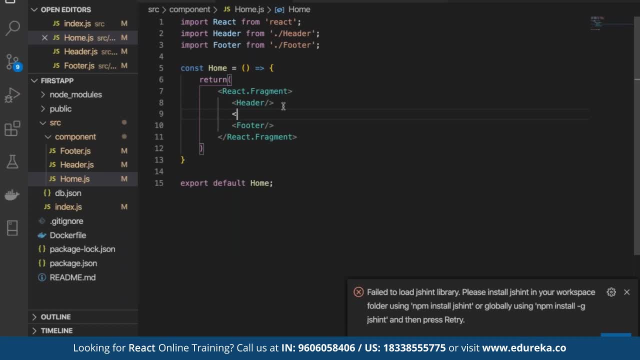 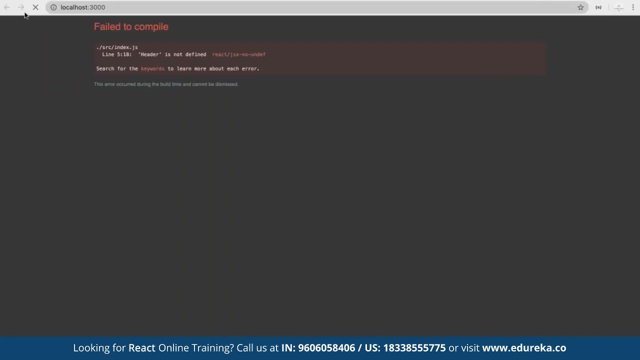 In between that I can write one. It's to tag and save home pages. Now I'll take this home to my index and render your lines. So, guys, we make a functional component and they look something like this: Let us efficient see you see home page, your header, your content. 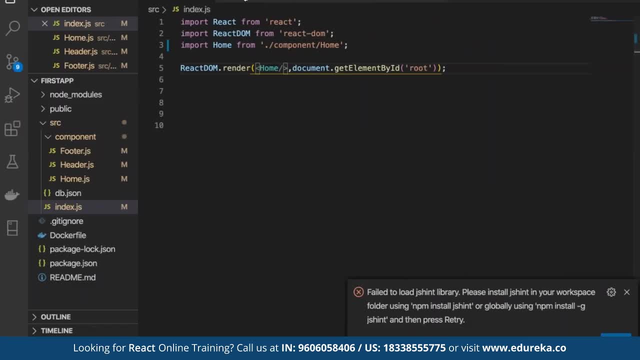 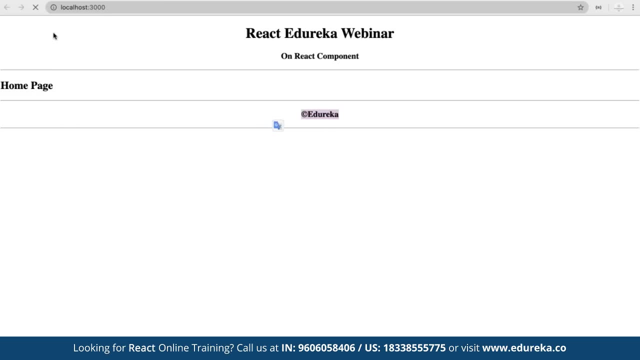 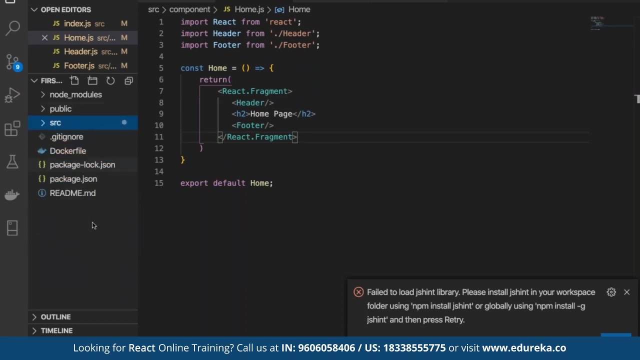 and your footer. So, guys, this is how exactly you define your component. It's called your functional component, Now how we pass a data. So you're not talking about the API right now. I'm talking about something else. I'm talking about something called as your state and props. 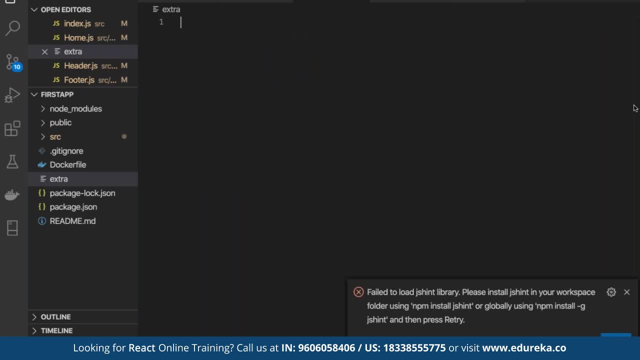 Let's understand that concept. It's very important to understand this concept of state and props. What is state? What is props? guys, every single component can have a local variable means. if I talk about only the first of all, the class-based comment can maintain state first thing. 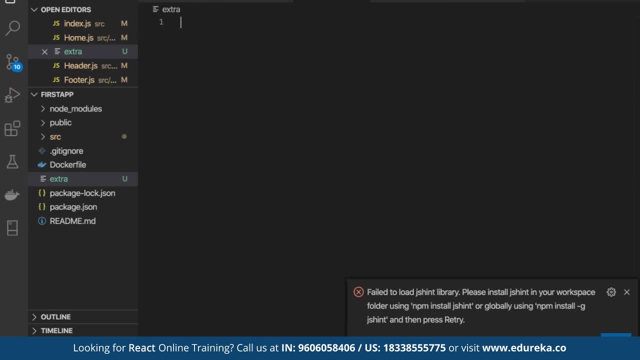 only class-based component can maintain state, So I can write: class component Can maintain state, So state. if our component a and component B, The state, act like a local variable, local variable, state is act like my local variable, every component have a state. suppose it our state, a state whose value. 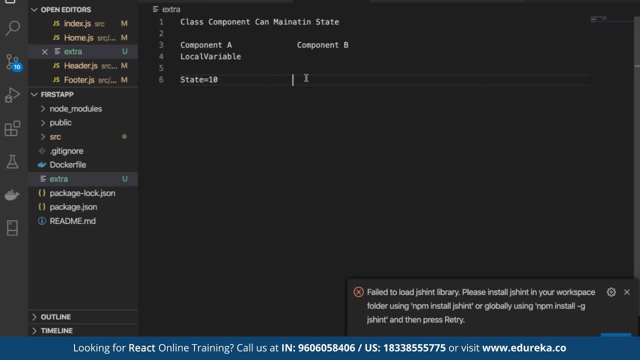 Is 10. component B: Have a state which is blank. state is like a local variable to a component. Now I want component a, that our state, whose value is 10, then our component B, that our state, which is blank. Now, if I want to pass a data from component a to component B, 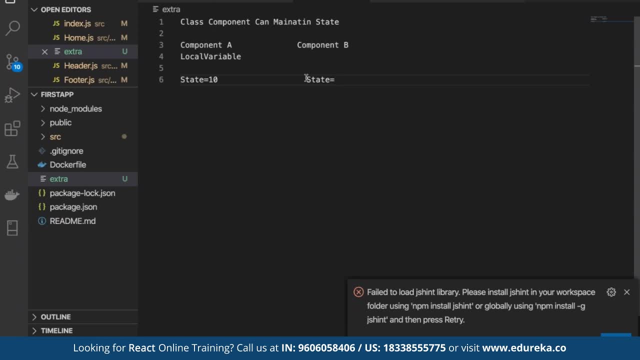 I will use props. I will use props. in short, I can say that every component can maintain its state and to pass a data between the component, we use props. and remember one thing: it can only happen in the case of your class. component means state can declare. 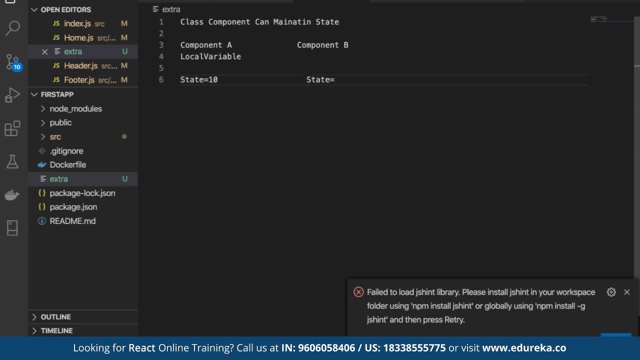 into the class-based component, but props can be used for a functional component. You have to pass a data to functional component. I can pass a data as a prop. The thing to learn here is that state is a local variable. prop is a way to pass up data. 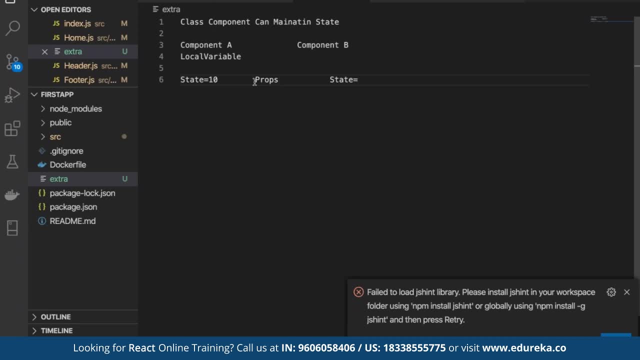 Let me show you a more practical. first of all, let's pass as a prop one thing as a prop. Now, if I go back to my component here, Say: home, okay, right If I write a tag, a HRU, right. 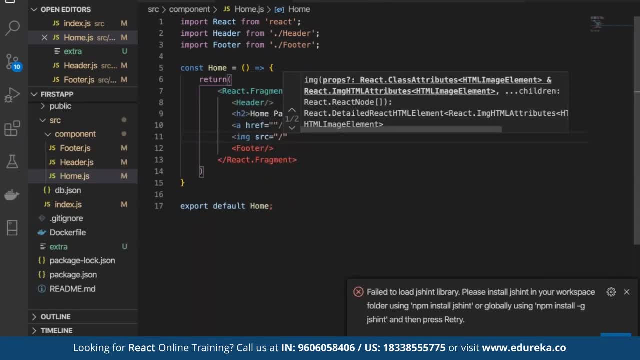 IMG, SRC, like that, Like this: now, what is your a HRF? What is your image SRC? Basically, HRF and the SRC, What are they? They are basically called as your attribute or our property. correct, They are basically refer as attribute. 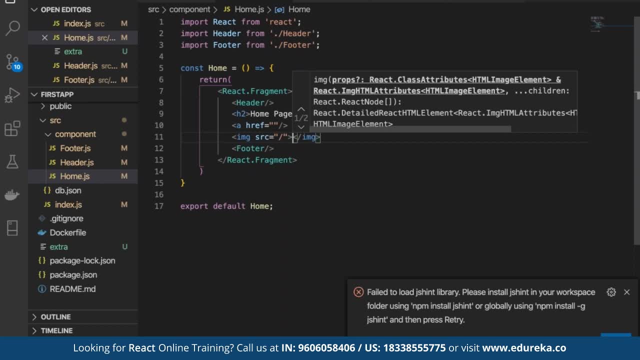 or a property of a component. In short, I can say that HRF and SRC is a property of a tag and image tag in a same fashion to my component. I can define a property how. let me show you. If I go here, footer, I write here: 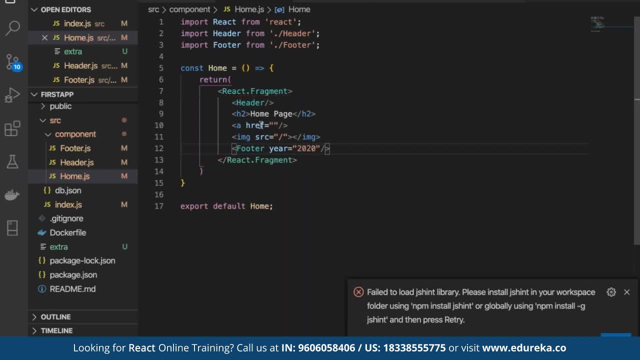 Okay, I write 2020, suppose, If you check this is a property, is a tribute with an is a tribute, its attribute and same thing its attribute. Now how the function component will receive it. in a functional component I can receive as a props: 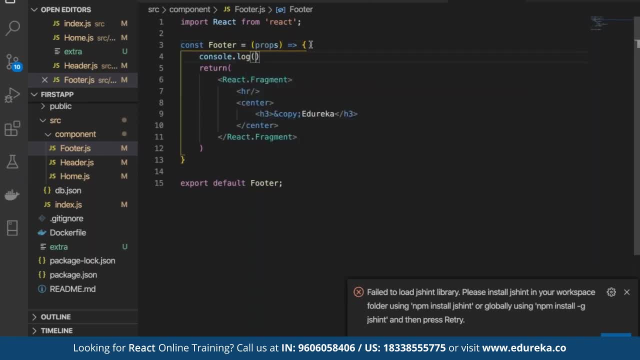 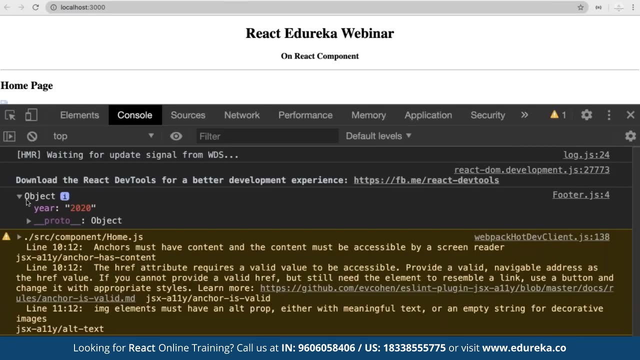 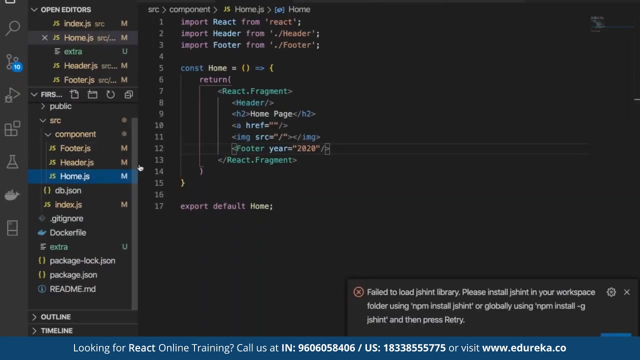 And I can write console dot log props. Let's see what we receive here In my footer, what I'll receive. I receive an object which have here as 2020 see. basically, I'm able to pass my data from home to footer, out to your props. 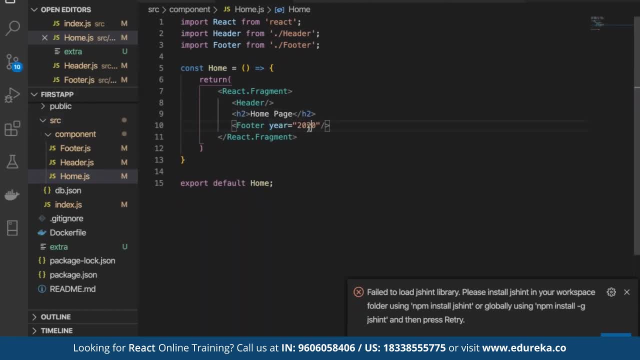 Through your props. here is our property to which we assign a value, and this value we receive in the footer at this place. Now, how do you use it? I'll simply bind it So double curly, single curly, bracket and write prop Dot here like this: go back to my browser. 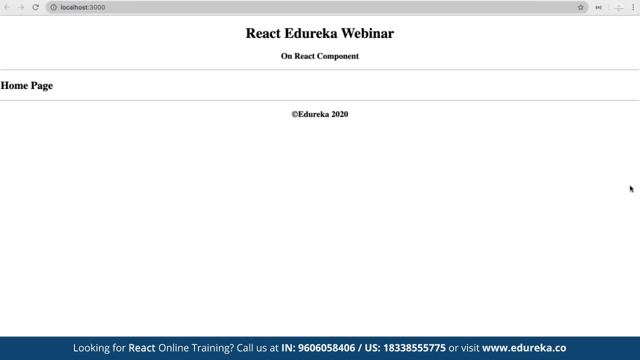 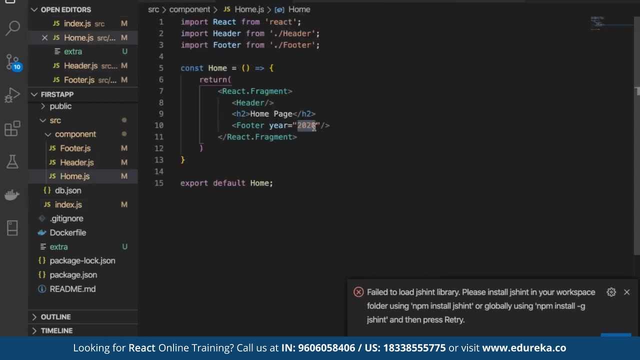 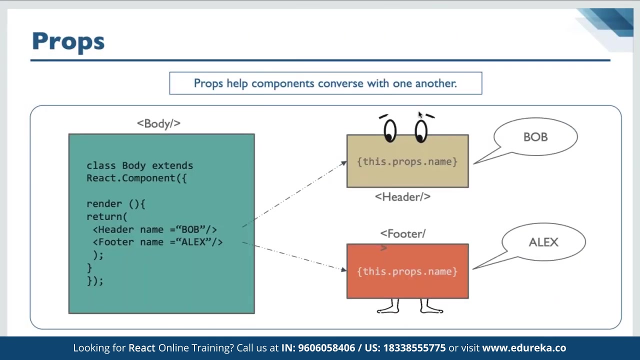 and check it, you see here: Edureka 2020.. Now, if I want to another property, if I change it, Next file, also home file, I'll make it 2021.. Now, see now video definition for that. So prop help to help component to converse with each other. 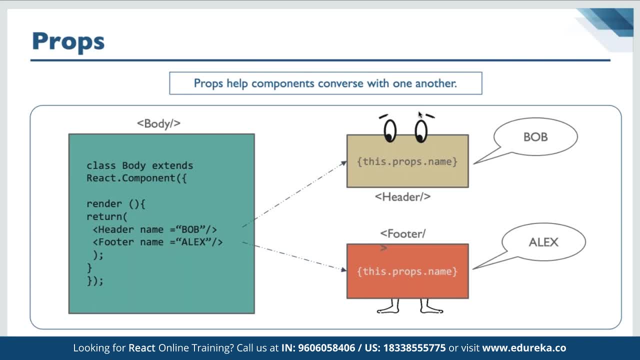 I said that prop is something which help to transfer data from one component to the component. then in one component We can pass multiple props. but right now these are understanding. I want to give you that what exactly or prop look like And what is state. 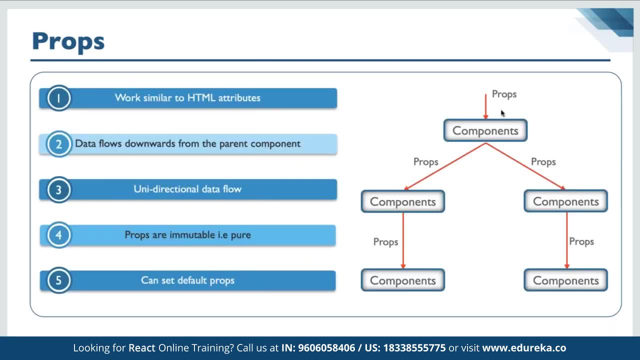 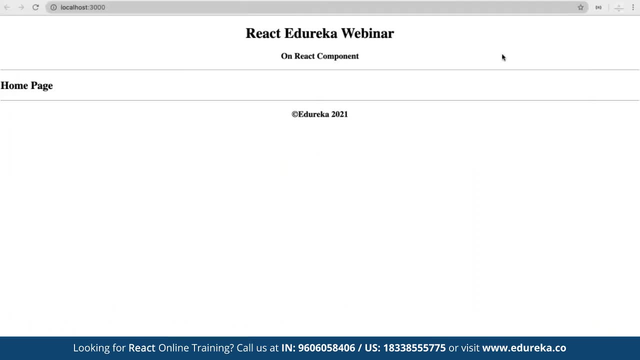 So we can pass the data from one component of the component. but the condition for that is it should be nested. It should be nested. nested means like this disco nested, One component, that other company, that is reference guys nesting. So comment should be nested when you pass a data. 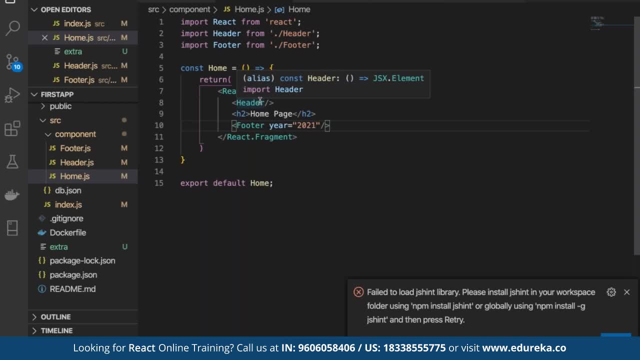 from one component to other company. Now let me show you how to make a class-based company. declare state this component. if I want to convert into class, Let me know how to make a class-based component For me. get class-based company. You have to import one more thing called as component component. 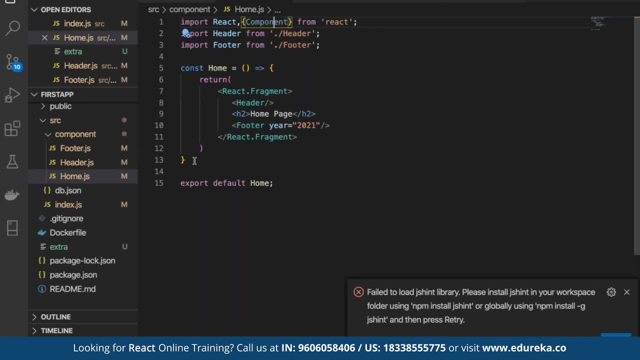 So to convert a same company to class base. I'll just put in a current command, So later you can see how we did that now. First of all, I use a keyword called class and right extends component and class cannot return inside the class to display the HTML. 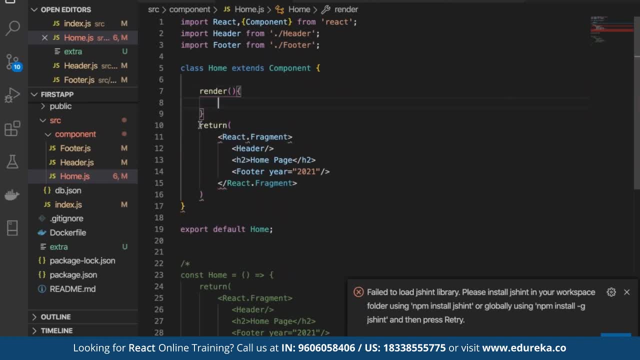 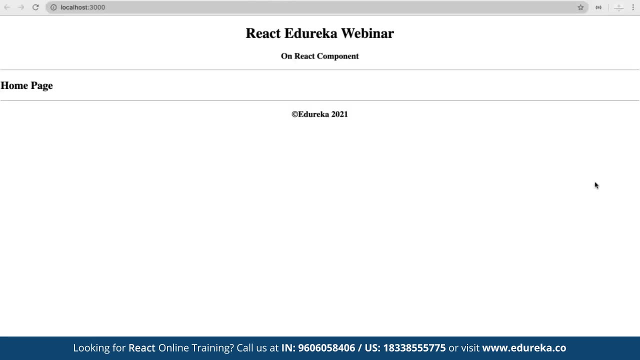 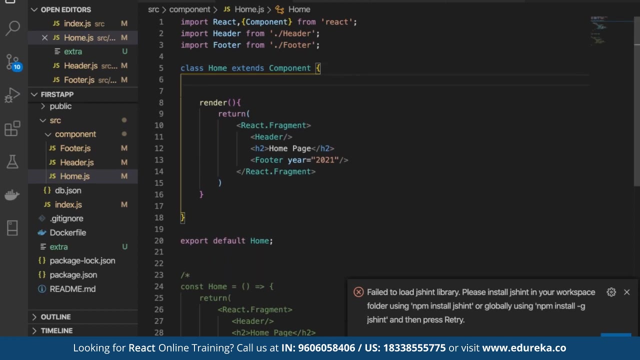 You will use render. render is a method that use inside the class to return the HTML. I guess it's look exactly similar right now, but ideally My company is now a classical How to get a state to declare a state: guys views, constructor, constructor inside the constructor. 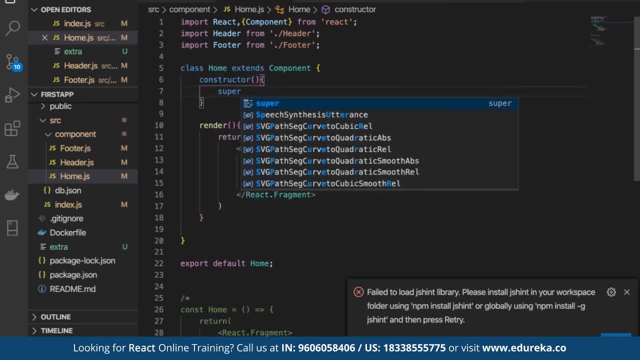 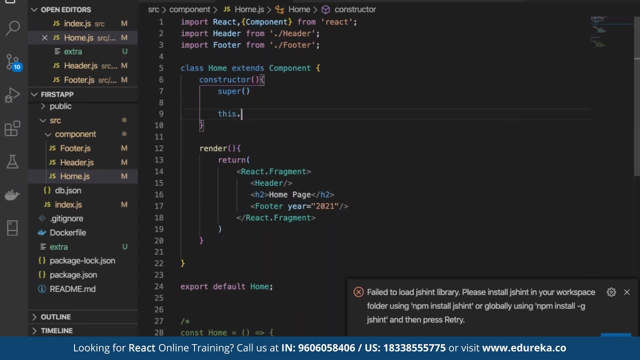 We have super keywords, super, and then inside that we can declare any state will write this dot state equal to curly braces and I can define a state variable. Suppose my state variable is heading, I'll say react and you data or say react webinar, simple. 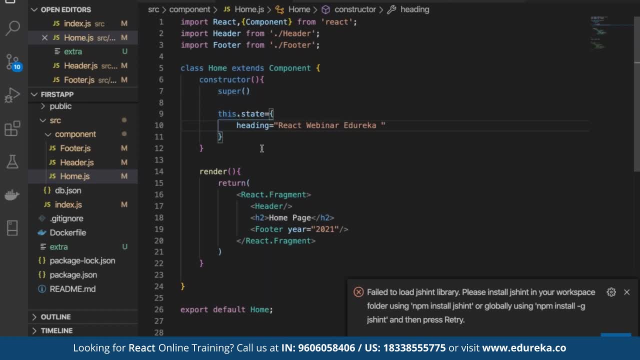 I want to do this now. This is my state. if I want to use a state inside a combine cell, Suppose, I'll say keyword, one more state variable, You can have defined multiple state variable, say keyword, as react course of that. If I want to just state inside the same component, 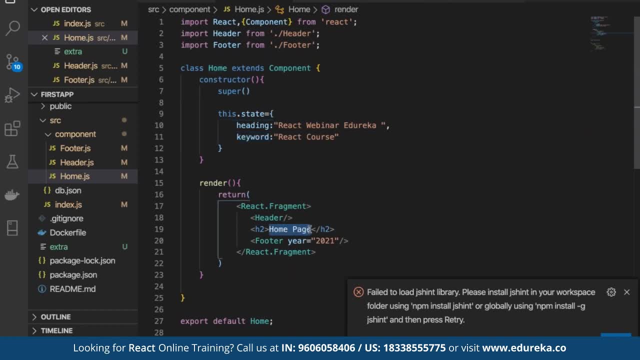 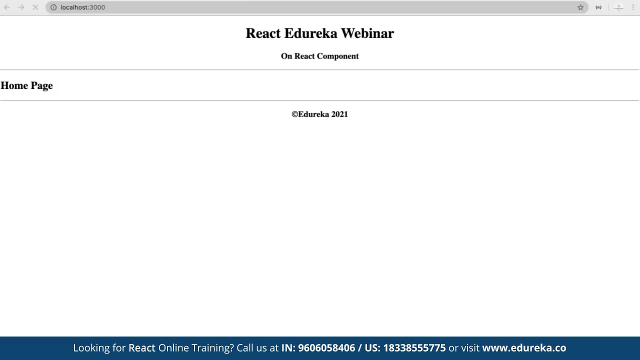 how to use it simple. I'll remove this under the curly bracket right. this thought: state dot state variable name. This thought state dot state variable name. that is keyword this. Okay, if you go back, let's see It's a react course. 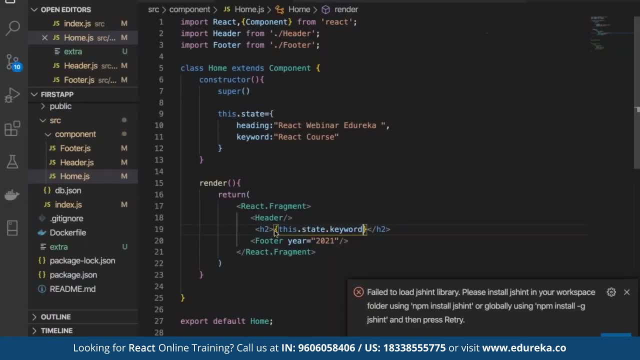 But if I want to pass this to next component, I can pass to header. suppose I'll say heading And heading I want to pass. I'll write this: dot state, dot heading. Now I can receive as a prop and display it in the header. 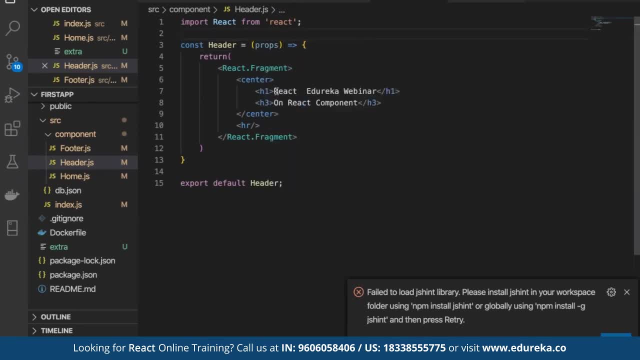 I'll receive that in the props, props dot heading, and I put a curly bracket and we'll say props dot heading. see a state of one component. I can pass to the again a class based component or to a functional component. That's what I'm telling you in the beginning. 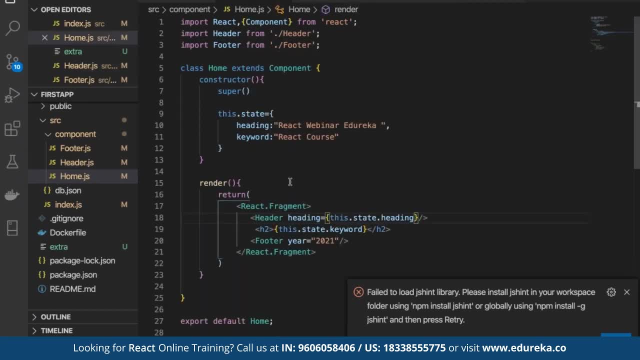 How is that can work is in my class component We call the API. So we can call the API here. Okay, and that API that we call, we get a data, We save the data in the state and that state we can pass to my component of function. 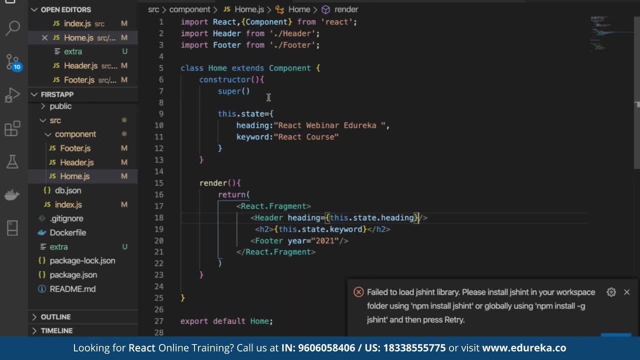 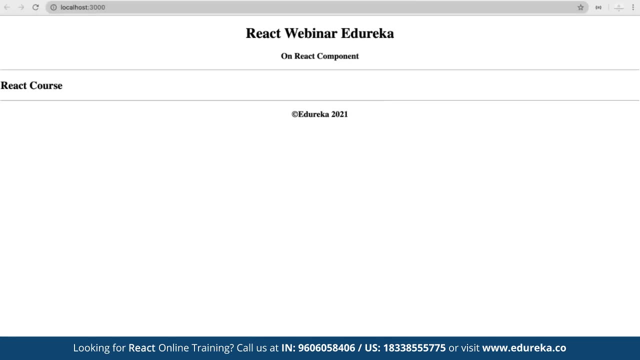 There are told a beginning. in the class component, We call the data with me I call, we define the state and in the function component we pass this data and pass at a state and on the screen we can see everything is working. Exactly similar. 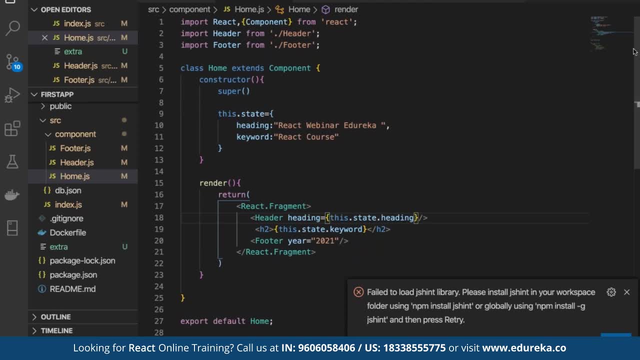 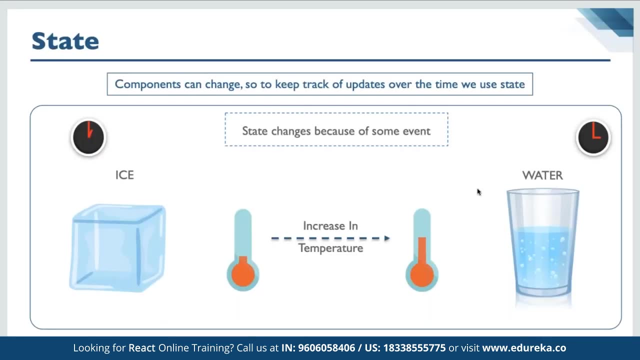 But now, once you can see very clearly how is that key data is transferred, Only show, know exactly passes, prop and the state component can change. So to keep the track of the update over the time, We can use state state change because of some event. 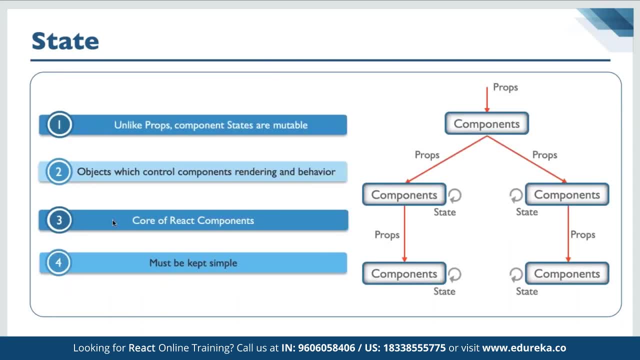 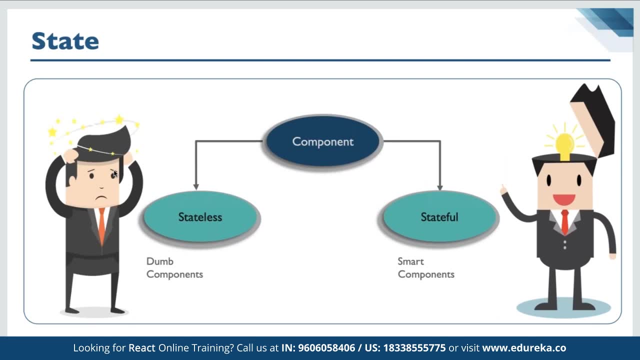 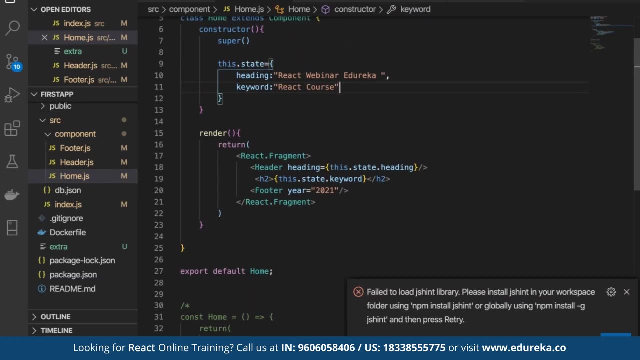 Increase in time and the basically object which control the competent rendering and behavior, basically anything about a combat. So now you understand Your class based company are called as a stateful company Why? because they can declare the state and the functional component are called dumb component. 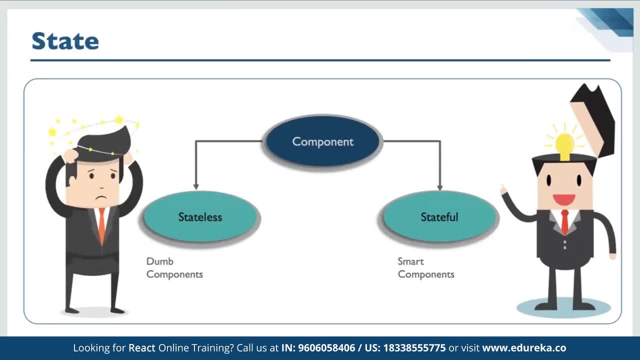 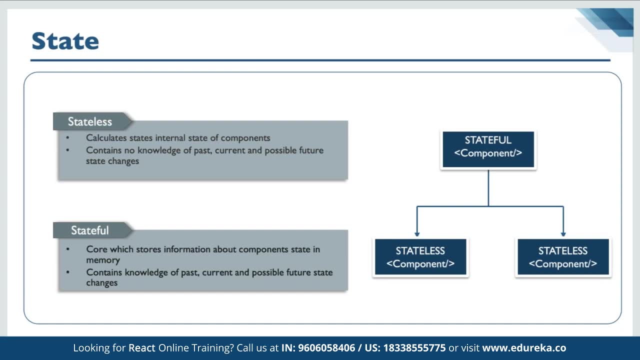 because they are stateless- Dumb component and smart component. stateless calculate state, internal state of a component and contain no knowledge of a past, current and possible state future. because we don't declare anything here, We don't save anything in a functional component. 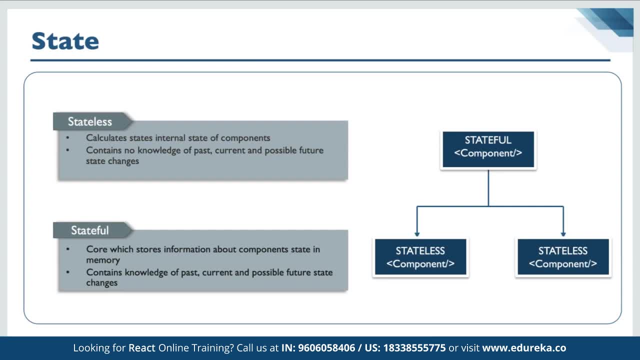 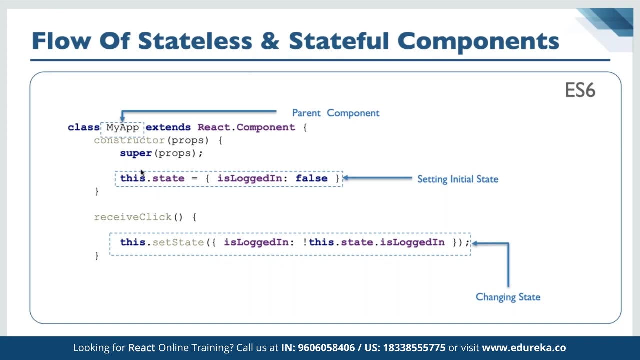 Where is Stateful core, which store the information about the component state in a memory and contain knowledge of past, current and possible future state? that's called your stateful companies. So I like a flow work. Basically, we can have our your functional component, class based component inside the class based component. 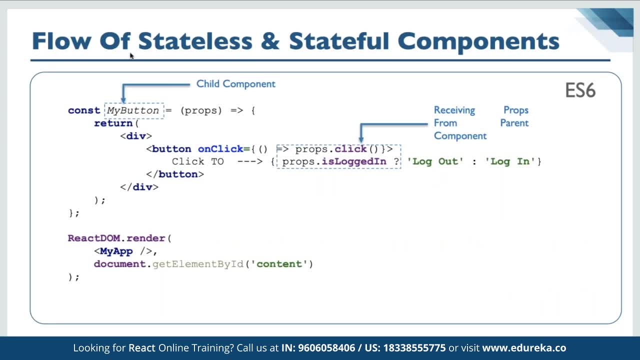 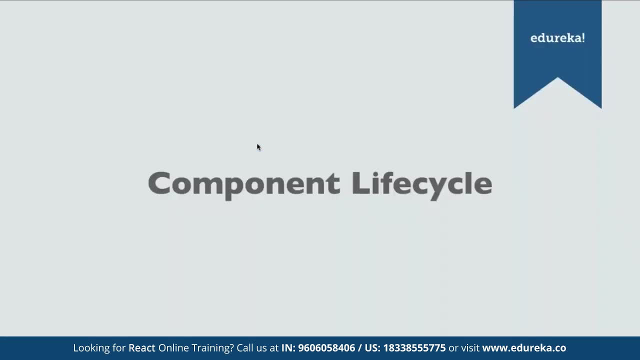 We call our functional component and we can pass the data from child to the functional. We already seen this thing right now. We already seen this thing right now, how exactly it works. Now one more thing I can add here. Basically, we can update the state. 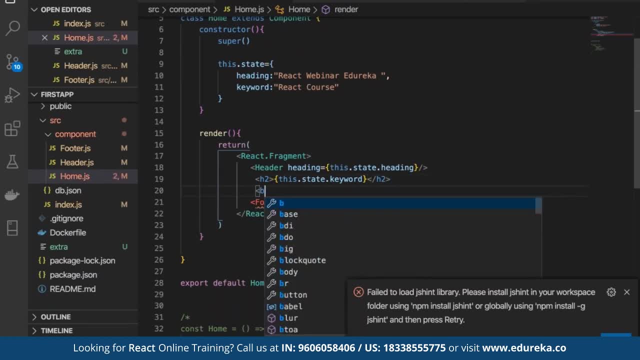 How suppose I want button here or simply date. I want input box Type equal to text. I want P tag here below this: I want whatever user will type, I'll bind it here. I want state called user input and say user input here. 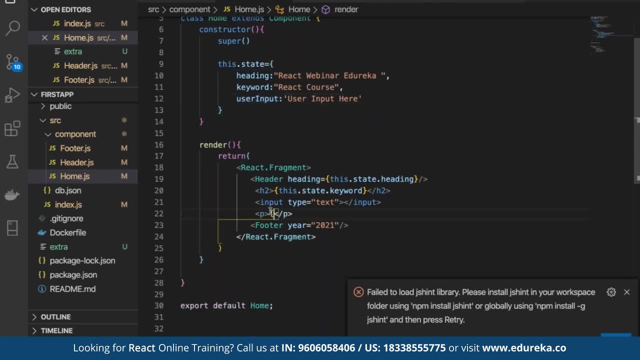 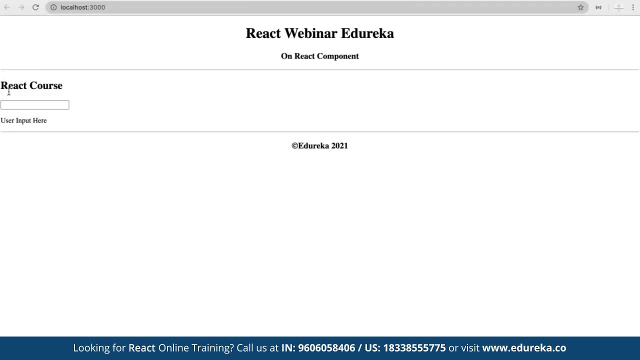 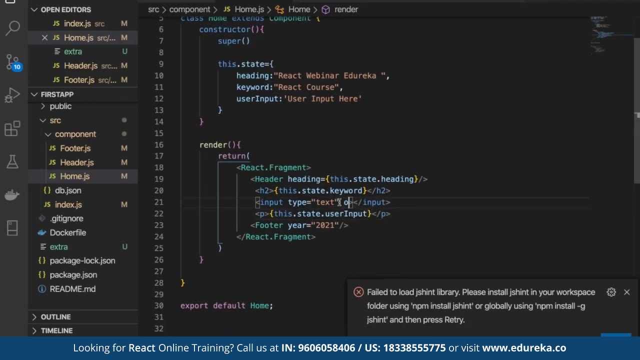 And this user input I'll bind initially. I'll say this: dot state, dot. user input. Go back right now. say I want, when users start typing something, I can show it below or we can do that. We can call an event. I'll call one events. it on change. 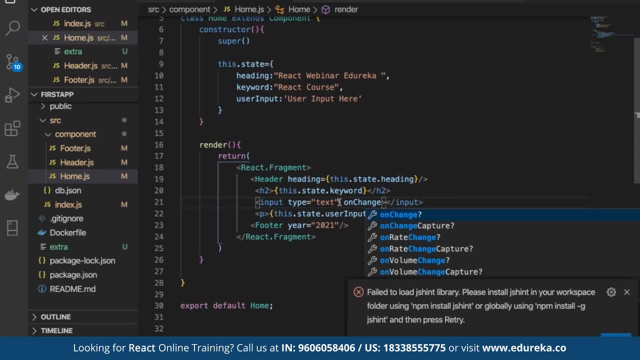 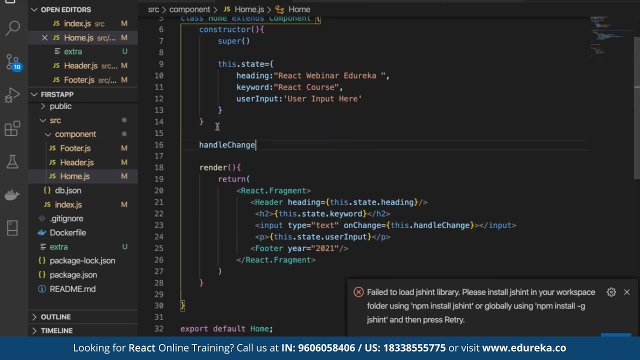 Basically on change. I'll call my comp: I function and change, update the state. How on change. I can call my function, say this thought and they'll change. Now this handle change. I can write here: It will receive one event Arrow: curly braces. 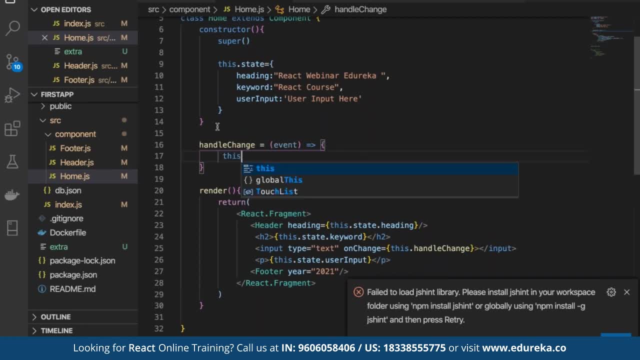 and we can call set state. is it this dot set state of what of my user input to what? what user is typing that will receive in event dot Target dot value. whatever, even got fire from there, I'll pick the value. So whatever user will type, I can update the state. 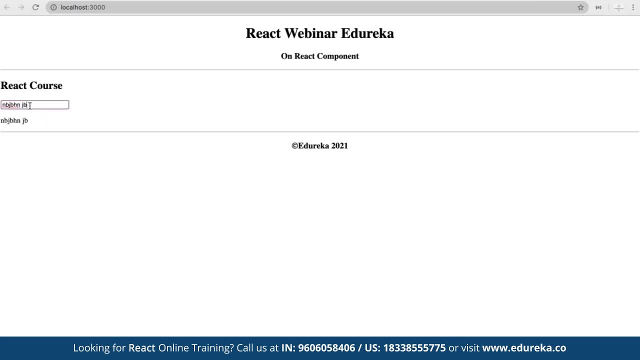 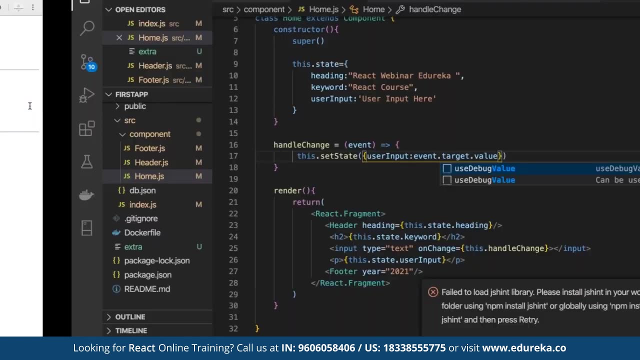 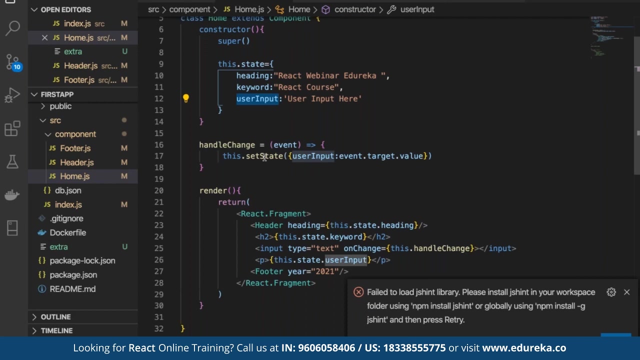 Let me show you. You see, whatever I'm typing, I can see it below exactly because we are setting the data in the state dynamically and binding the state. that is basically reference, guys. You're updating a statement for that use set state Now, as last topic of our session, that is, component life cycle. 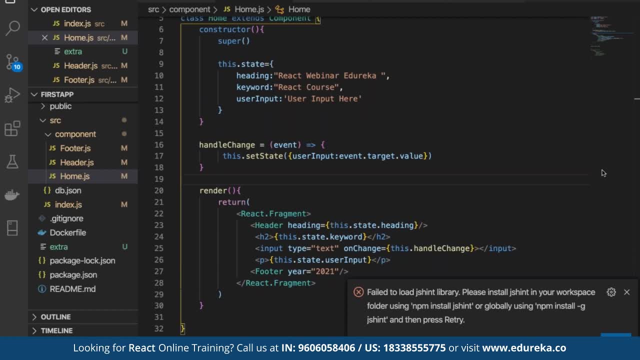 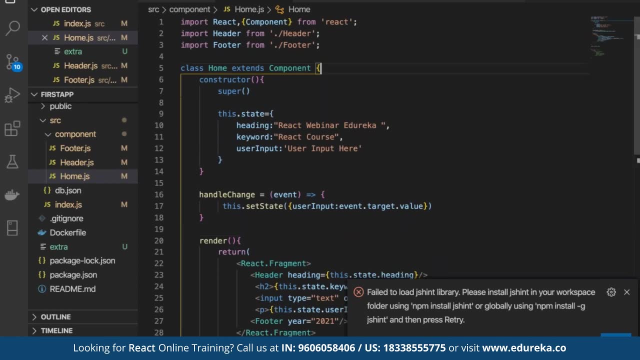 Basically what happened whenever the component load. we have to control the flow of a component. Right now, for some of my component, I'll show you how that life cycle work. life cycle is work basically how exactly your component. render means which part run first, which part run next. that's called life cycle. 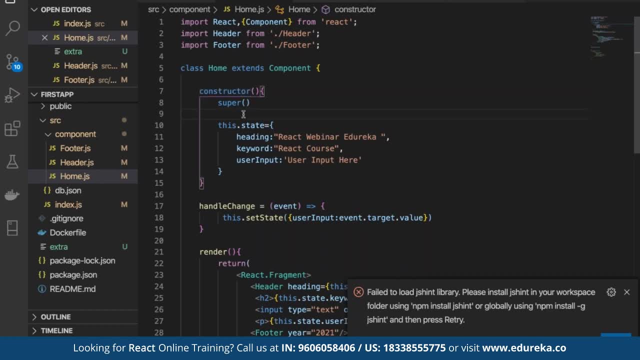 In any component of a class, the Constructor is always the first thing that get called. It's not about the JavaScript in about any class in a Java, Python, Ruby, whatever you pick, The very first thing that you run is always your Constructor and consolelog inside Constructor. 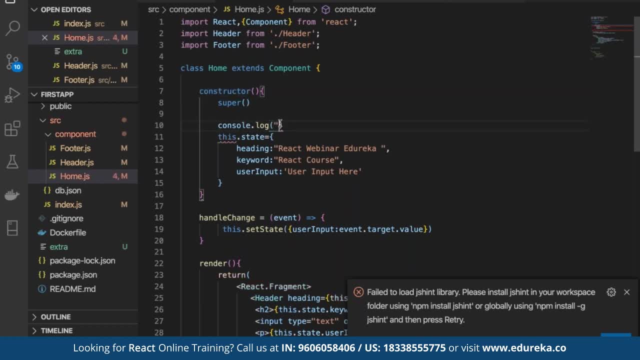 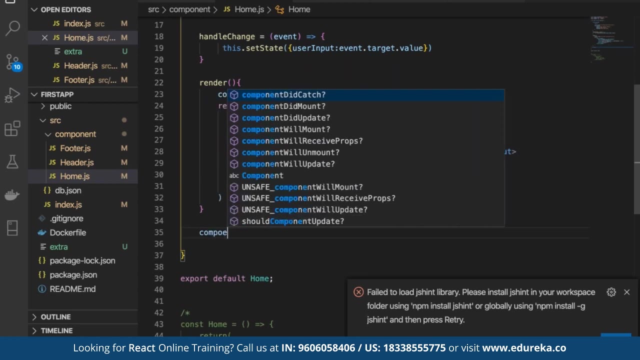 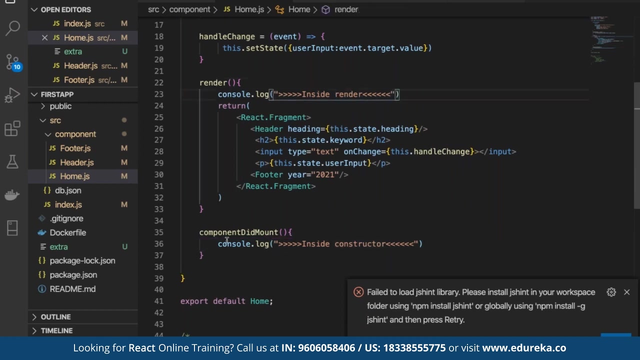 just to show you how exactly it looks like. And then I write render. this I'm life cycle. Look, I'll write only one in this demo, The one thing called component did Mount. there's so many, but we'll talk about one. and we write inside render, inside comprehended Mount. 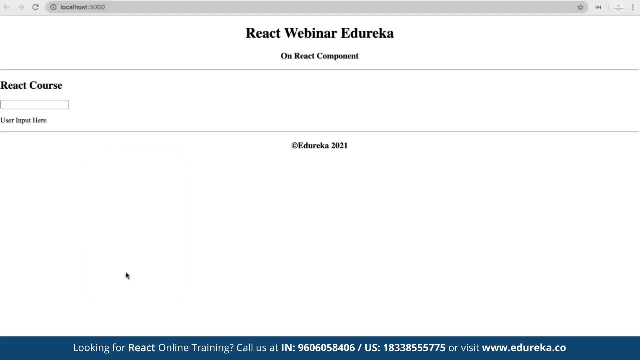 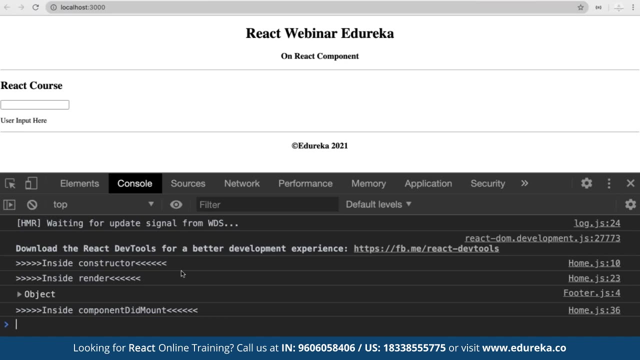 So if I render this, if I inspect this, I'll show you. basically, guys, the very first thing that get called inside that class is always your Constructor- see Constructor get called. after Constructor, the render get called and after render competent did Mount get called. So if I want to declare anything, all the declaration I'll do. 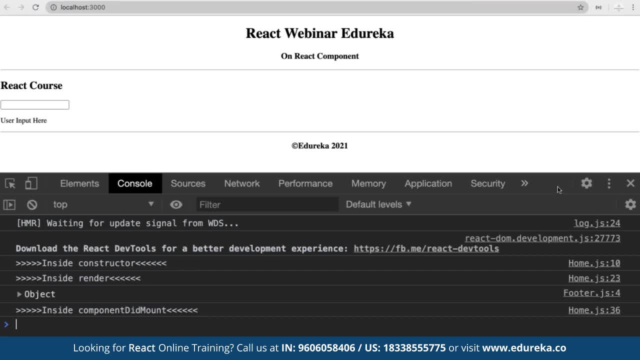 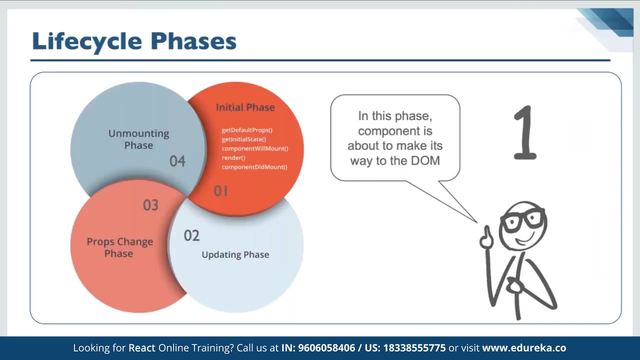 inside the Constructor And after Constructor you will go inside the render and after render will have competent did Mount, did Mount is something that run after and all your API calls You will do inside it, Mount. So I'll talk about some more composite. first stage is called initial phase. 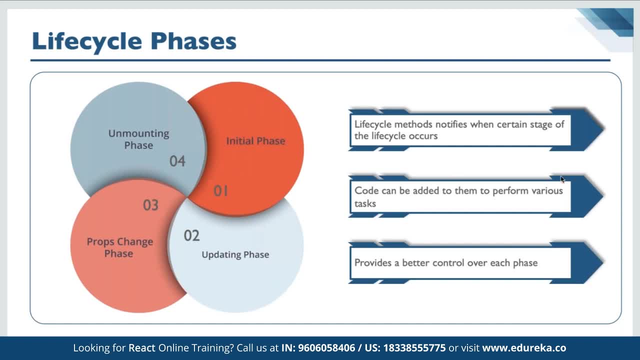 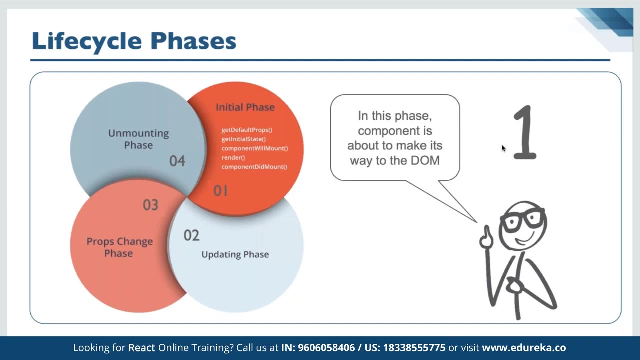 initial phases, very. declare the state into the Constructor. That's called initial phase. Okay then next stage is called this: updating state. First of all, component declare: Inside this stage, stage competent is about to make a way to the dorm. the very first stage of a component. 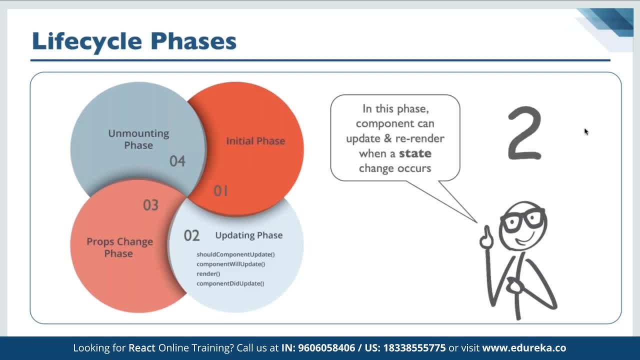 And the multiple life cycle called inside the stage. second stage, called updating phase. in this phase competent can update and render when a state change occur. So ultimately, in this phase competent can update and rerender when the state change occur. third, called prop change. In that prop change particularly what exactly happen. 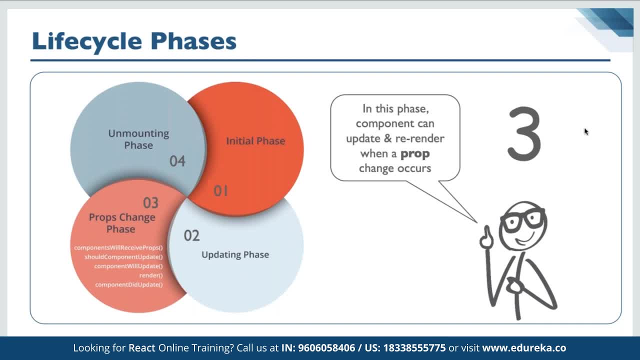 is in the prop: change competent, update and rerender. Remember one thing. I'll tell you a basic funda. whenever the state change happen, Remember one thing: your competent will rerender. Okay. whenever the state change happen, competent will rerender always. 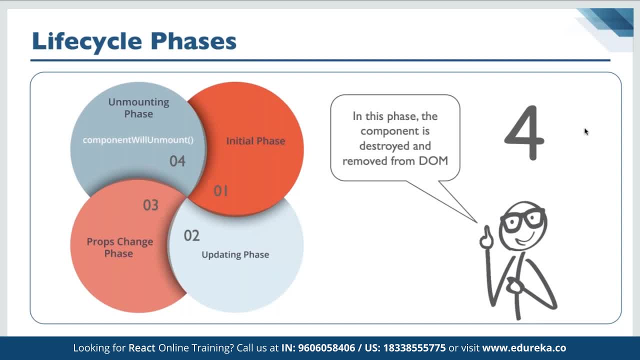 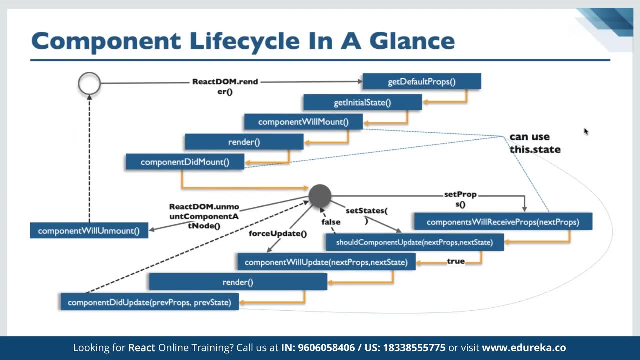 So in the third phase, competent will state will update and then the competent will rerender again. then there are multiple life cycle. are present days like: get default prop, get initial state, competent will Mount render, did Mount competent will unmount and then competent will receive props should comment update. 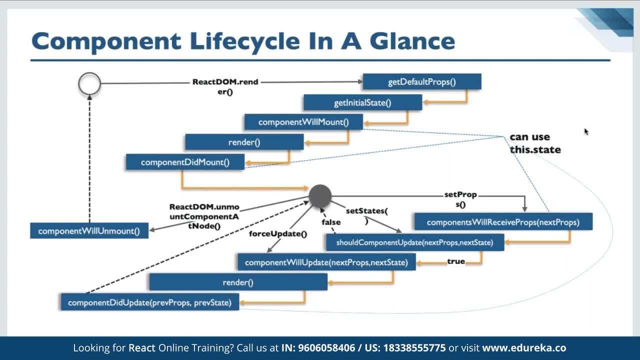 competent will update, render competent, update, like that. So ultimately, there are multiple life cycle hooks. ultimately, the point is like that: You need to know that in more details. Okay, so this is, guys, how exactly your life cycle And the component work. Cool guys.